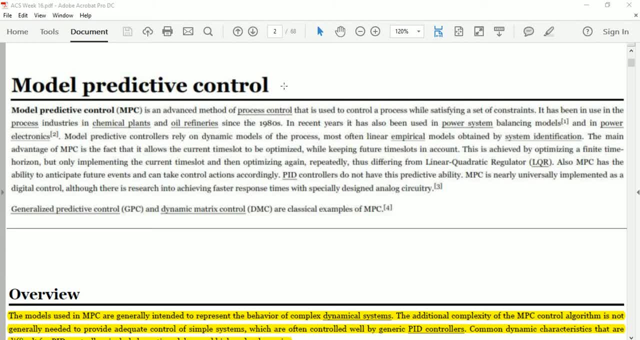 Then it also has a predictive ability, that it predicts the future. It also has an observer. we will see its algorithm. now It can predict, ie it has predictive ability. So, looking at all these things- MIMO system, predictive ability and set of constraints- 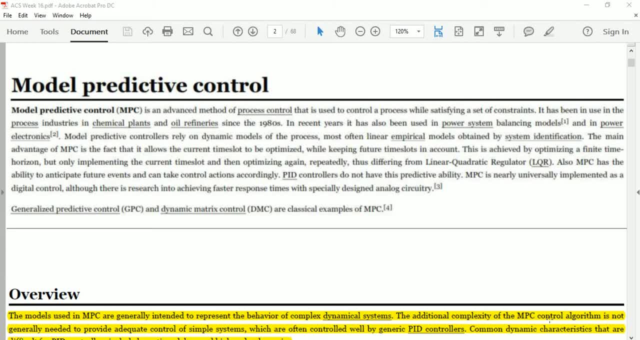 looking at them. this controller works and because of this it becomes a very powerful controller. It has been in use in the process industries, in chemical plants and oil refineries since the 1980s. In recent years it has also been used in power system balancing models and in power electronics. 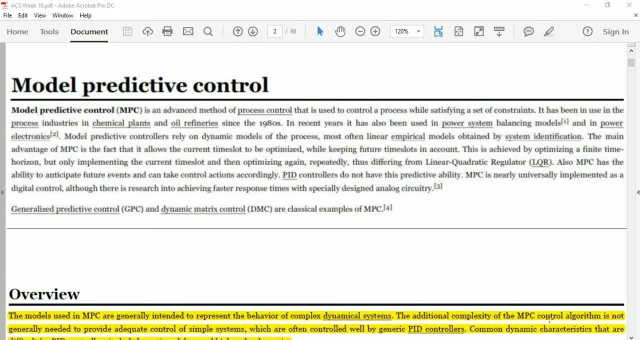 Model predictive controllers rely on dynamic models of the process, most often linear empirical models obtained by system identification. So we have already discussed system identification in previous lectures. The main advantage of MPC is the fact that it allows the current time slot to be optimized while keeping future time slots in account. 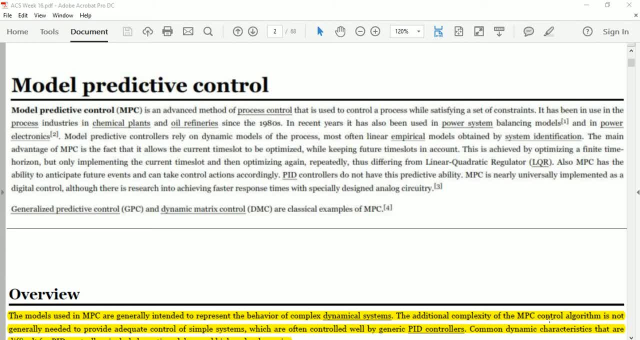 We will see in the next equation that this is achieved by optimizing a finite time horizon, but only implementing the current time slot, ie it will work in its current time slot, Then optimizing again, or it will repeat this process further in the next step. 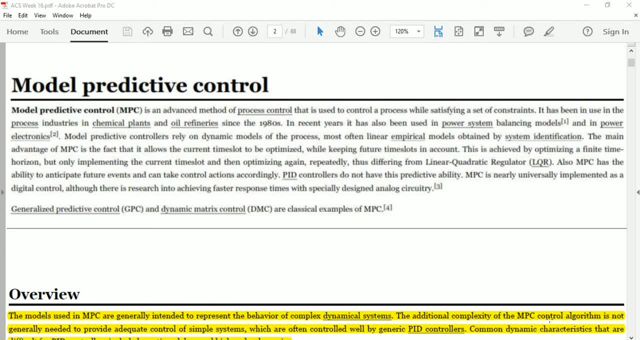 Repeatedly thus differing from linear quadratic regulator. Also, MPC has the ability to anticipate future events and can control actions accordingly. PID controllers do not have this predictive ability. MPC is nearly universally implemented as a digital control, although there is research into achieving faster response with specially designed analog circuits. 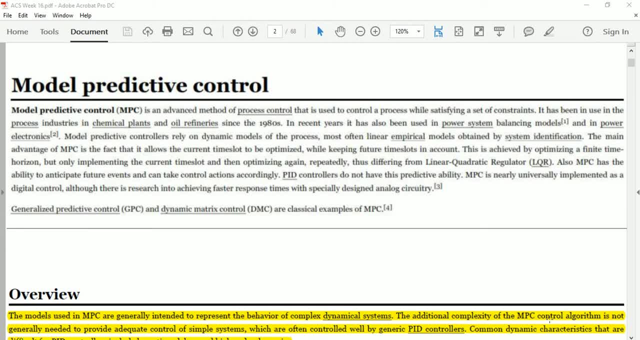 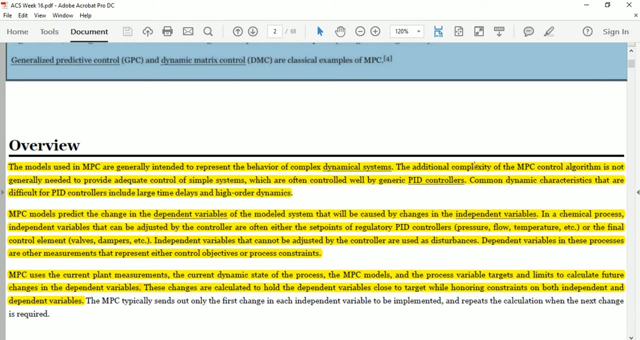 Its two forms are generalized predictive control and dynamic matrix control. These are the two popular forms of MPC. In this lecture we will take the idea of MPC. How does MPC work and what is it? The models used in MPC are generally intended to represent the behavior of complex dynamical systems. 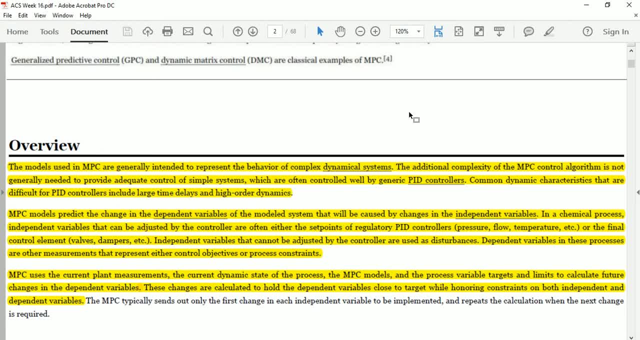 The additional complexity of the MPC algorithm is not generally known. It is only needed to provide adequate control of simple systems, which are often controlled well by generic PID controllers. We use it for these complex processes. Common dynamic characteristics that are difficult for PID controllers include large time delays and higher order dynamics. 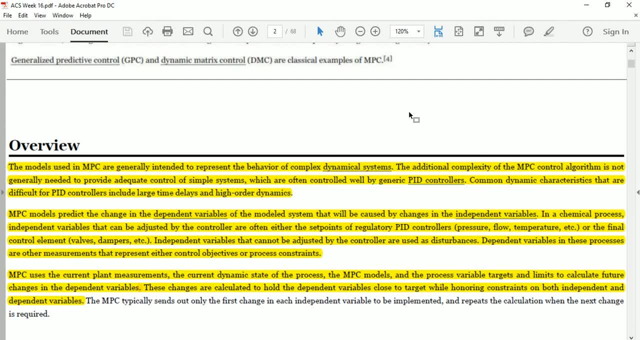 MPC models predict the changes in the dependent variables of the model system that will be caused by changes in the independent variables In a chemical process. independent variables that can be adjusted by the controller are often either the set points of regulatory PID controllers, pressure flow, temperature or the final control elements. 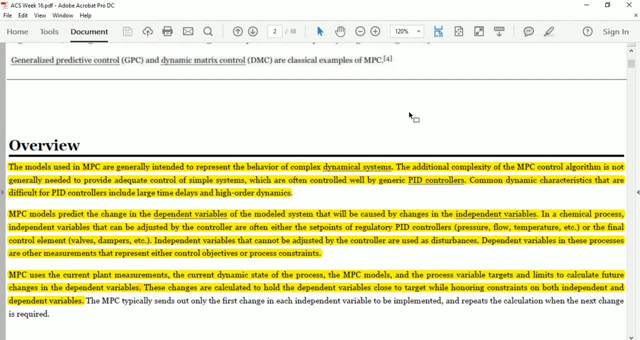 Independent variables that cannot be adjusted by the controller are used as disturbances. Dependent variables in these processes are other measurements that represent either control objectives or process constraints. MPC uses the current plant measurements, the dynamic state of the process, the MPC models and process variable targets and limits to calculate future changes in the dependent variable. 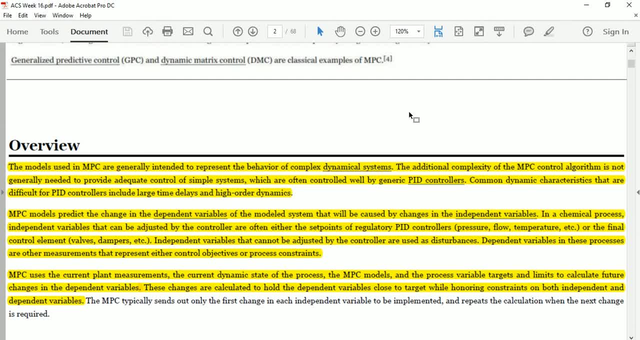 These changes are calculated to hold the dependent variables close to the target while honoring constraints on both independent and dependent variables. See what is in this. You will achieve the set point and respect the constraints. The MPC typically sends out only the first change in each independent variable to be implemented and repeats the calculation when the next change is required. 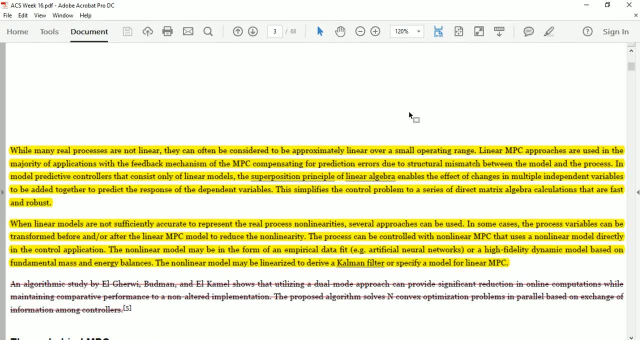 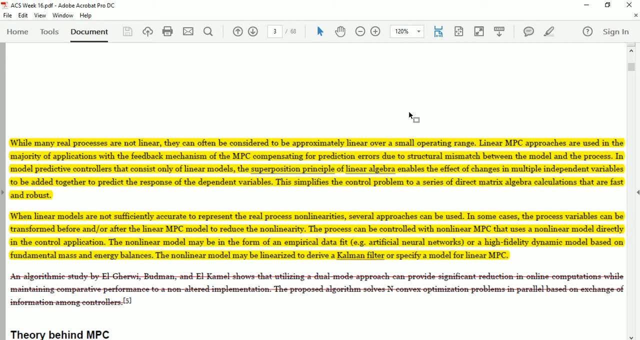 It will perform its work at every step. While many real processes are not linear, they can often be considered to be approximately linear over a small operating range. We have already discussed this in the linearization video. Linear MPC approaches are used in the majority of applications, with the feedback mechanism of the MPC compensating for prediction errors due to structural mismatch between the model and the process. 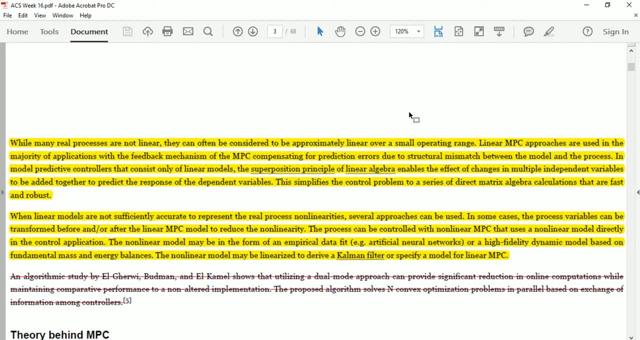 In model predictive controllers that consist only of linear models. the superposition principle of linear algebra enables the effect of changes in multiple independent variables to be added together to predict the response of dependent variables. This simplifies the control problem to a series of direct matrix algebra calculations that are fast and robust. 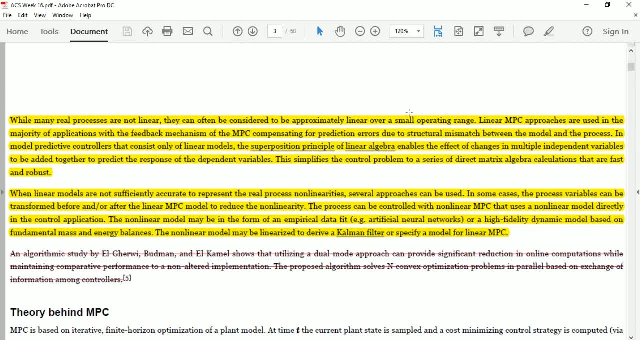 When linear models are not sufficiently accurate to represent the real process non-linearities, several approaches can be used. In some cases, the process variables can be transformed before and or after the linear MPC model to reduce the non-linearity. The process can be controlled with non-linear MPC. 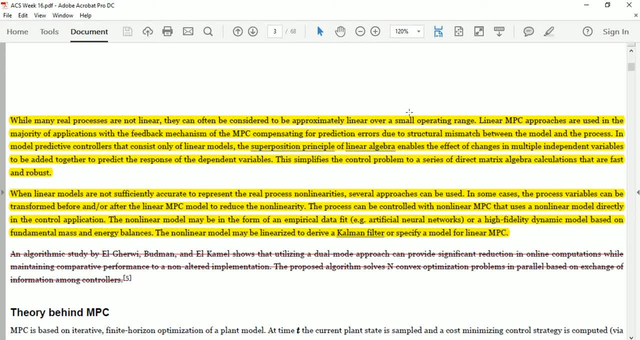 The MPC that uses a non-linear model directly in the control application. The non-linear model may be in the form of an empirical data fit, For example, artificial neural networks. We have discussed this in the last lecture on artificial neural networks. We use an empirical model based on data. 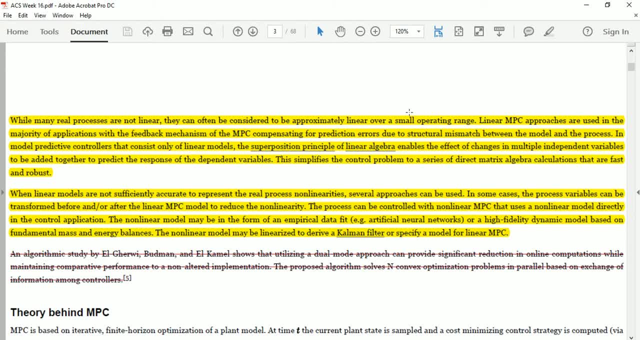 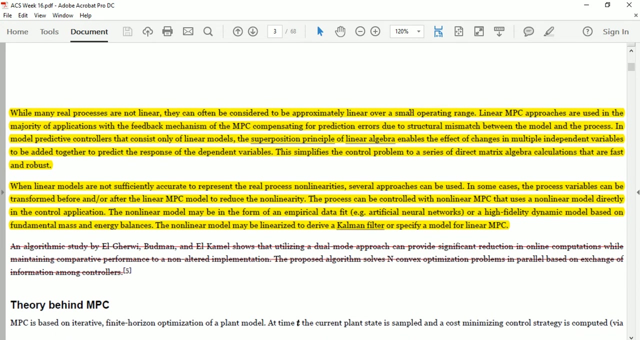 And a high fidelity dynamic model based on the fundamental mass and energy balances. The non-linear model may be linearized to derive a Kalman filter and specify a model for a linear MPC. The Kalman filter can be used for estimation. The MPC is based on iterative finite horizon optimization of a plant model. 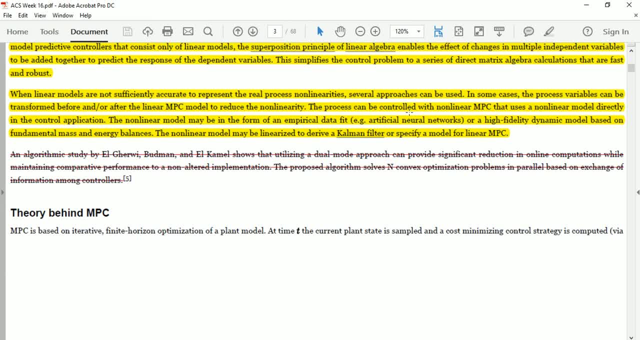 The MPC is based on iterative finite horizon optimization of a plant model. The MPC is based on iterative finite horizon optimization of a plant model. At time t, the current plant state is sampled and a cost minimizing control strategy is computed. At time t, the current plant state is sampled and a cost minimizing control strategy is computed. 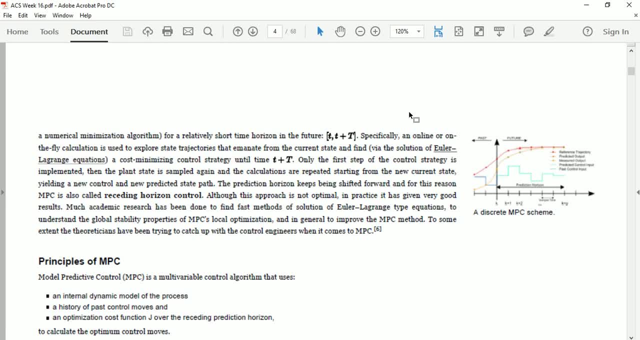 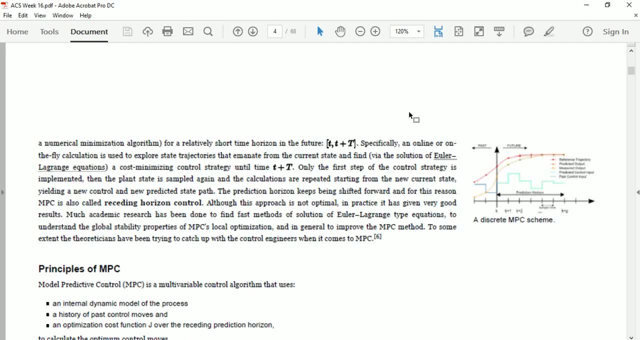 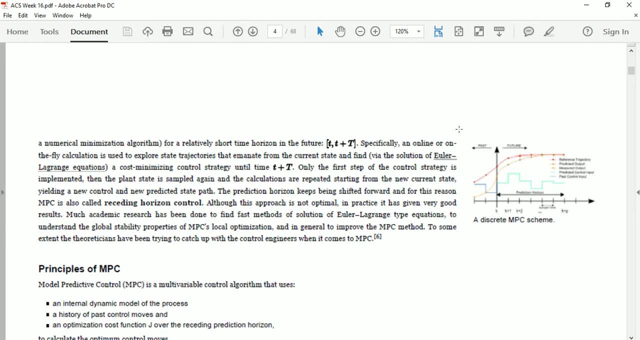 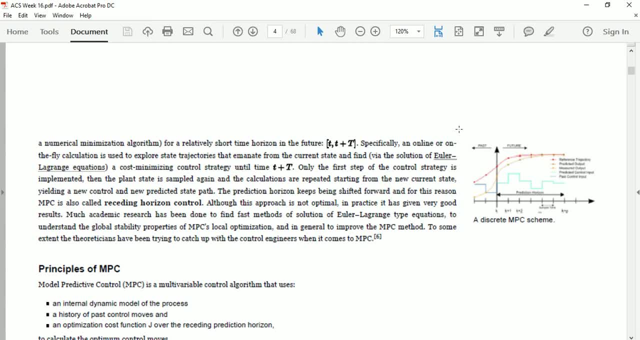 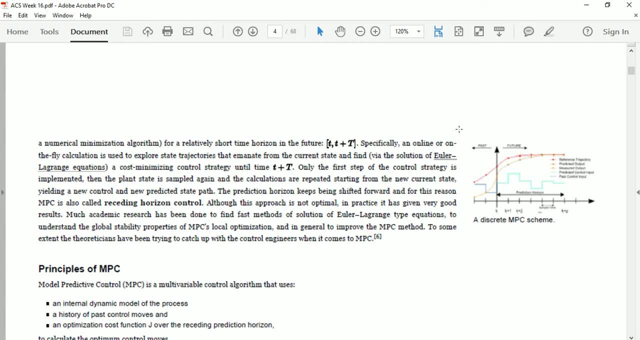 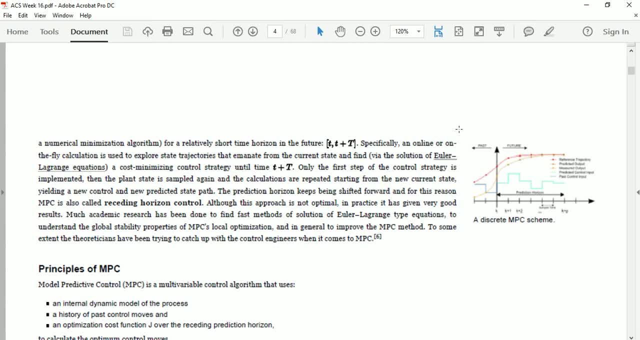 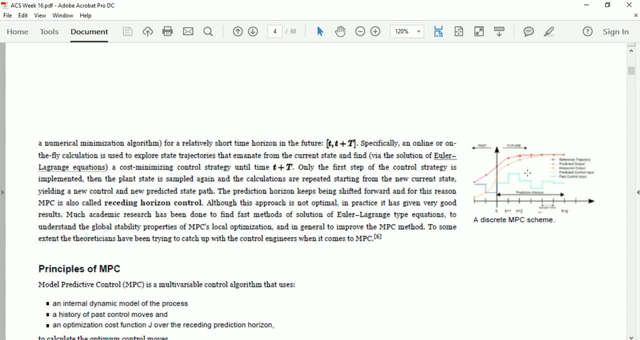 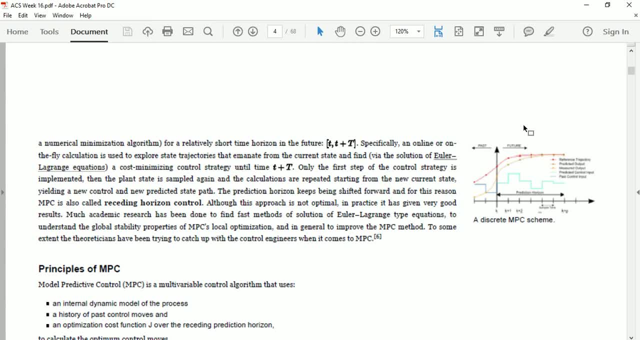 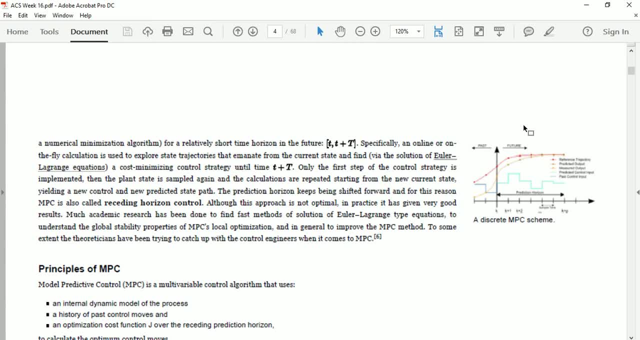 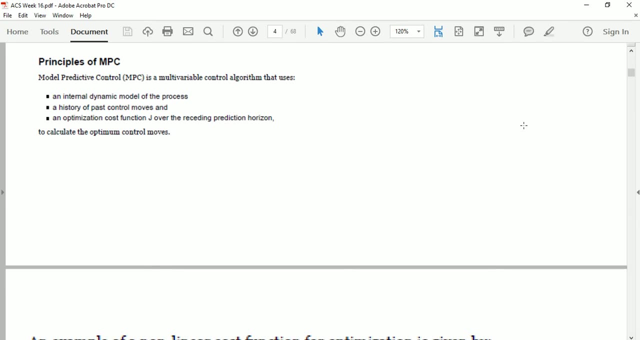 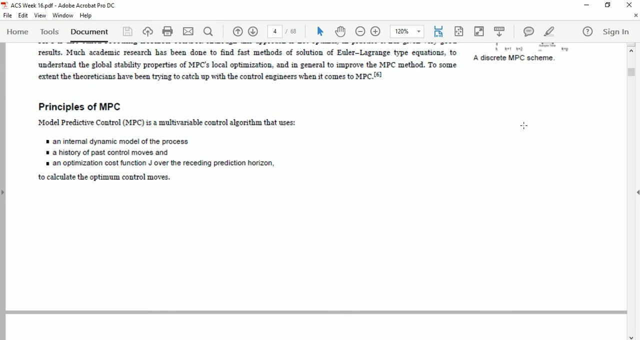 understand the global stability properties of MPC's local optimization and, in general, to improve the MPC method. to some extent, the theoreticians have been trying to catch up with the control engineers. What are the principles of MPC Model predictive control is a multi variable control algorithm that uses an 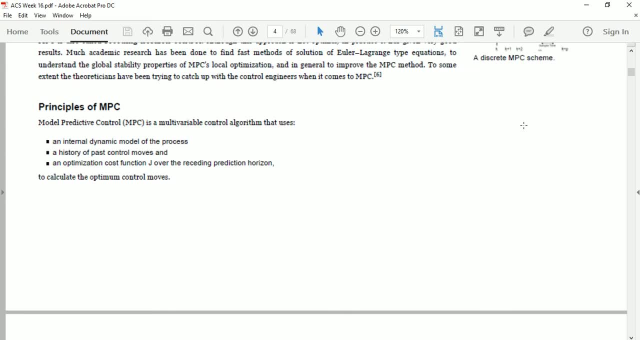 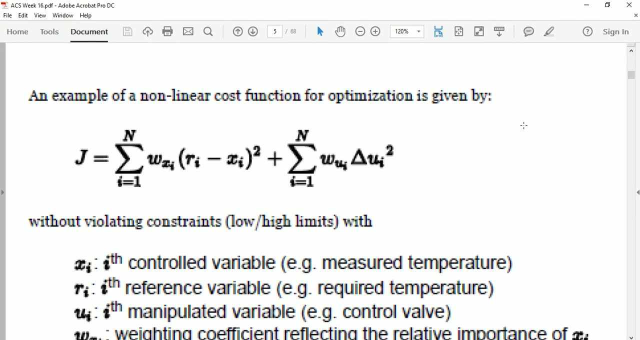 internal dynamic model of the process, A history of past control moves and an optimization cost function over the receding prediction horizon to calculate optimum control moves. 1200-500,000 squared is thesergeant limit for the self-assструментal simulation. 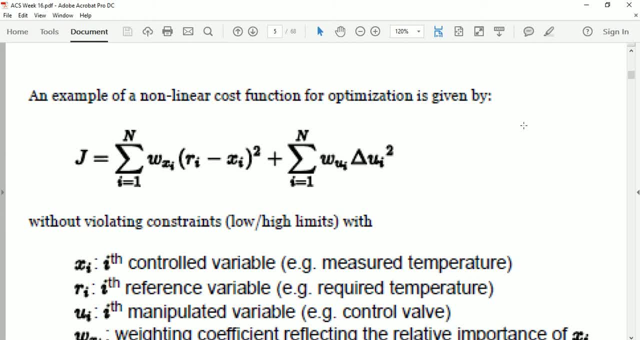 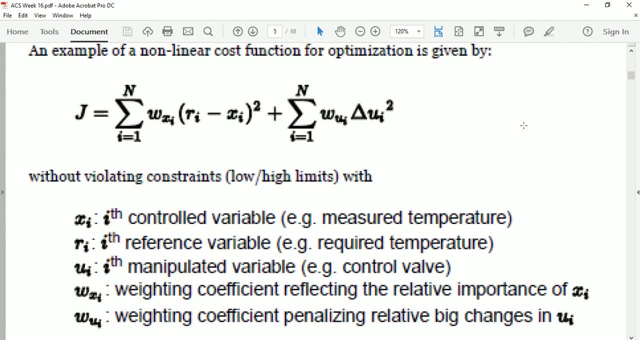 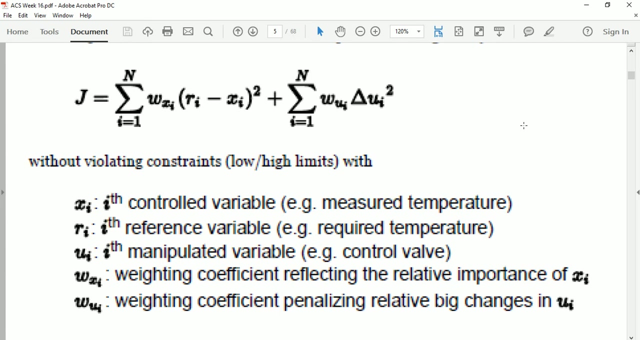 The standard estimates are as follows: j log, jjjjj, plus summation i2 equal to 1 up to capital N, w into Delta u i square. okay, now see, in this you have defined your limits, that you are optimizing and you are staying within the limits of your inputs and outputs. 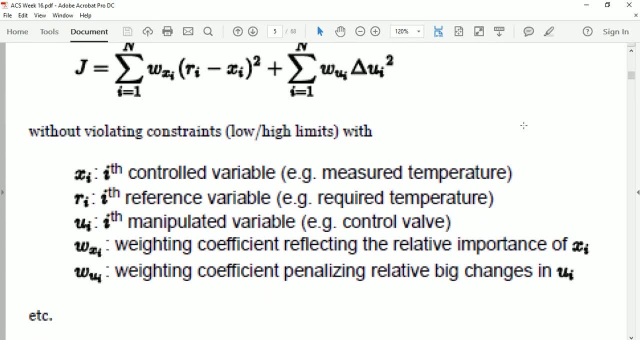 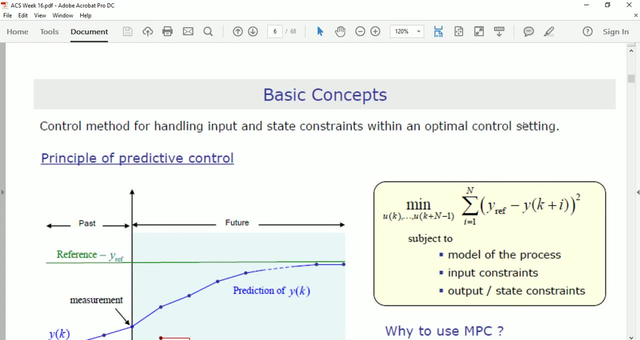 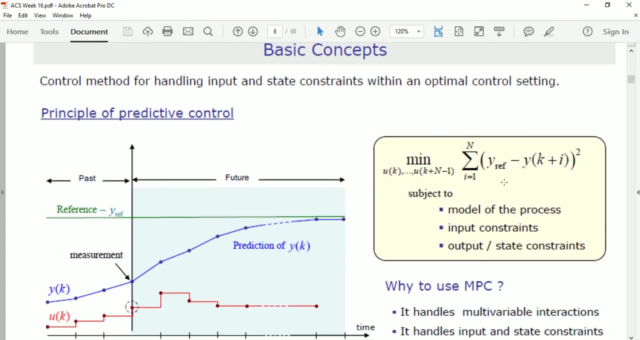 you have defined it within the limits now, after this control method for handling input and state constants within an optimal control setting. now see this will be more clear. minimize is a cost function. minimize i equal to 1 up to N y, reference minus y of k plus 1. k plus i, overall whole square. 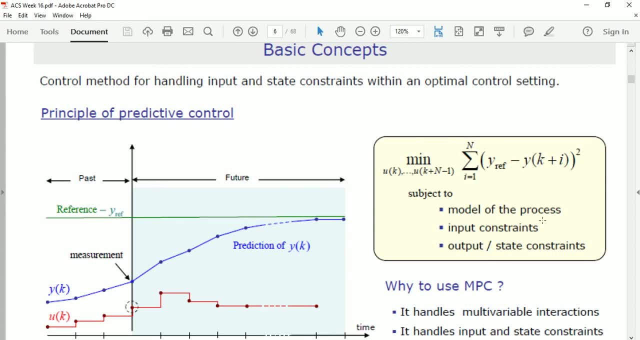 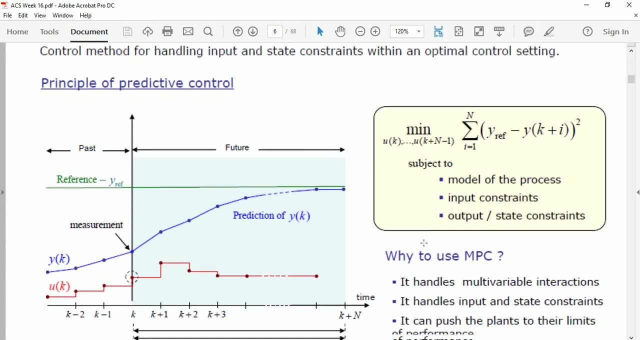 subject to the model of the process: input constraints and output state constraints. you have involved these constraints in this, and this is your past, this is your present and this is your future, or receding horizon control will be called like here: it will work and calculate this, then it will reach here. 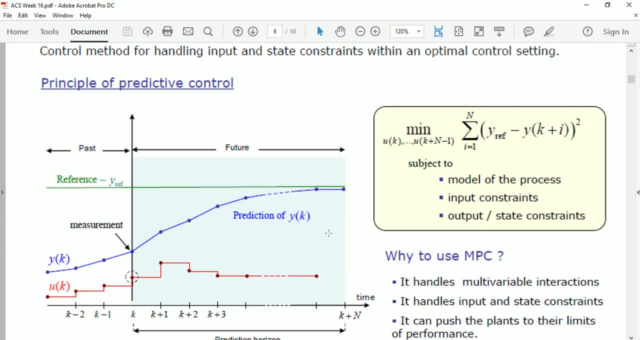 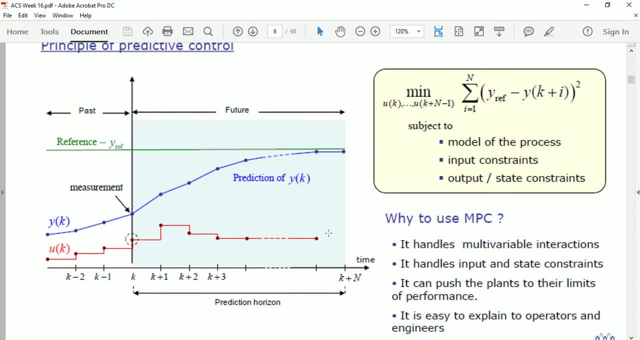 then it will calculate this, then it will reach here, then it will calculate further. okay, it handles multivariable interactions. it handles input and state constraints. it can push the plants to their limits to the performance. this is very important point: it can push the plants to their limits of performance. 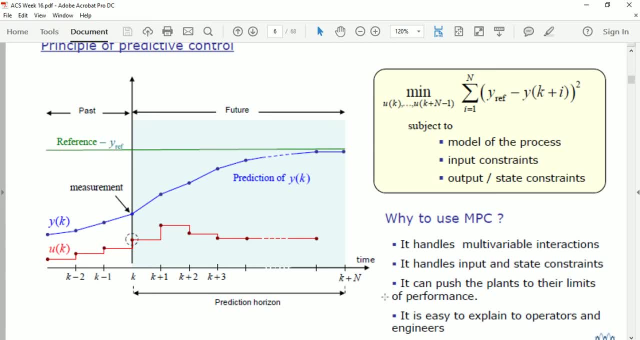 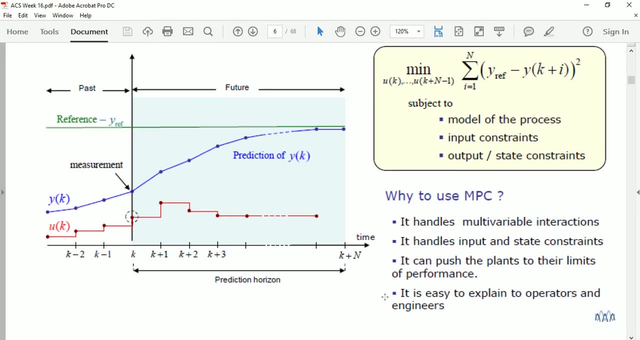 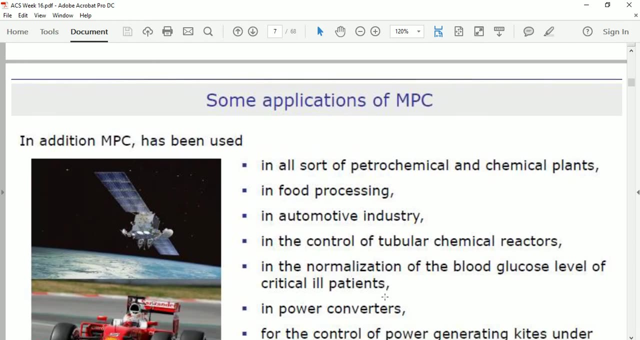 ie the limit which can be maximum, which can be matured, the process which can be matured, maximum it can be matured. so it is easy to explain to operators and engineers. okay, now let's see. so what are its applications? in addition, MPC has been used in all sort of petrochemical and chemical plants. 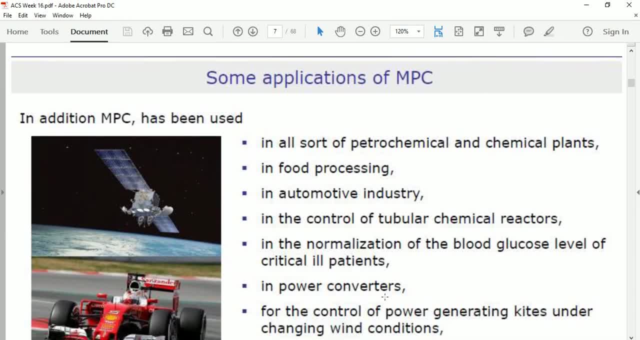 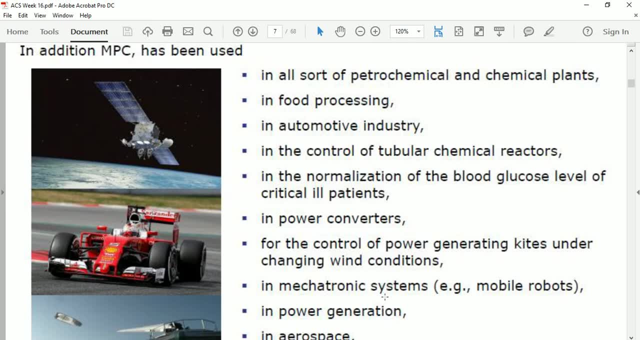 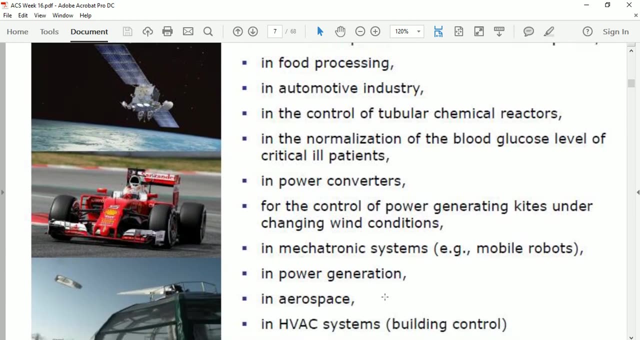 in food industry, automotive industry, control of pubular chemical reactors in the normalization of the blood glucose level of critical ill patients. in power converters for the control of power generating kits under changing wind conditions. in mechatronic systems, mobile robots and power generation, aerospace and hvac applications. 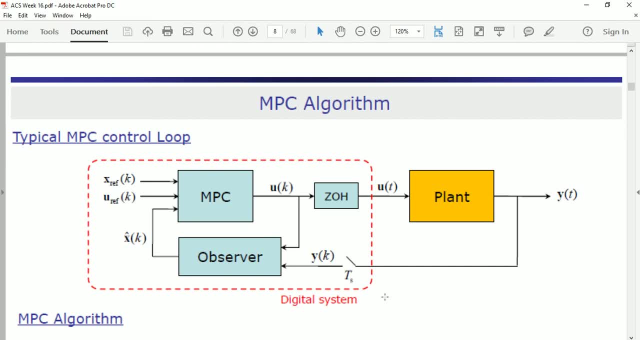 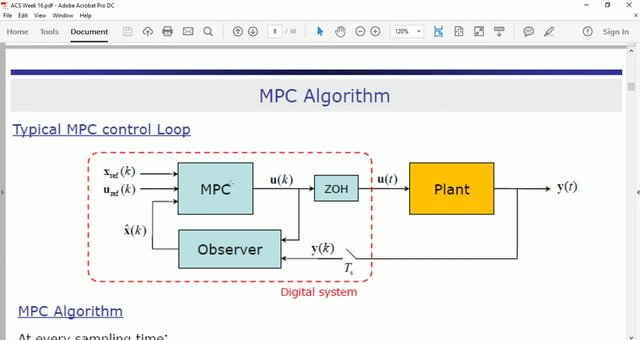 and it is used in all of them. okay, see, this is a control loop of typical MPC in which you can see that MPC controller is installed. optimization algorithm is installed in it. okay, after that its output came out of controller which is called UK input to the plant. 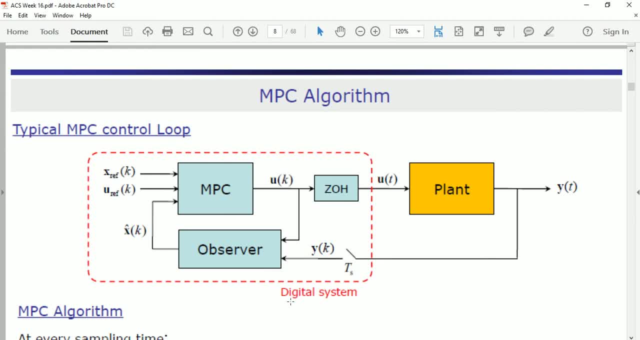 input to the plant after that, because it is a digital system, so the diagram of digital is made in it, in which zero order hole is installed, in which this digital to analog conversion is made with zero order hole, sample and mold. we will call it zero order hold. 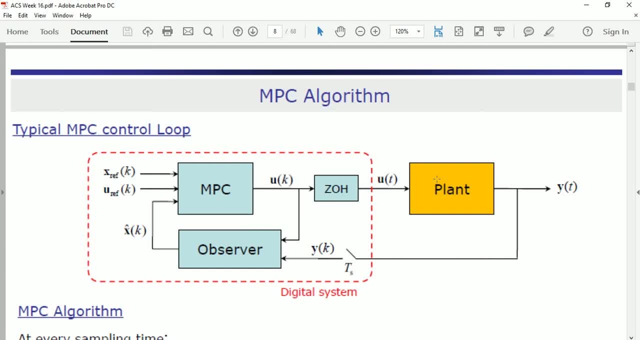 here zero order hold is made, analog is made and analog output will be digitized. sampler is installed. after that, now see this observer function came. observer is the parallel model of the plant. so in this you see that the input you are giving to the plant, you will give the same input to the observer. 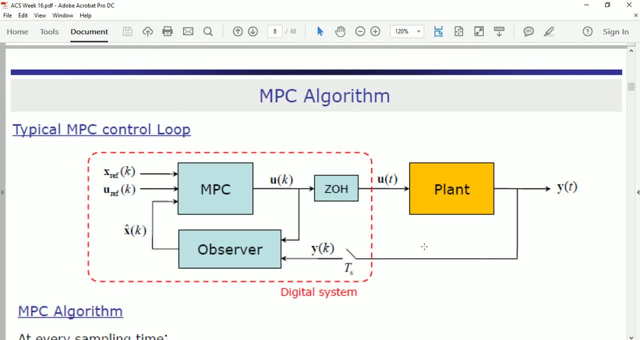 and the output of the plant is also given to the observer and then from both of them its estimated state. you are developing an estimation of x of k and inputting it. that is the same prediction prediction you are doing from here. from this observer, you will generate the prediction y of k plus 1. 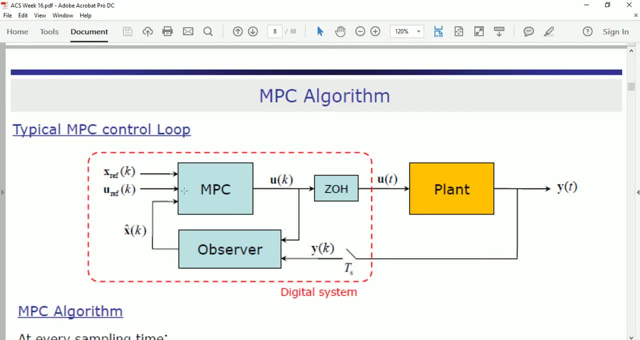 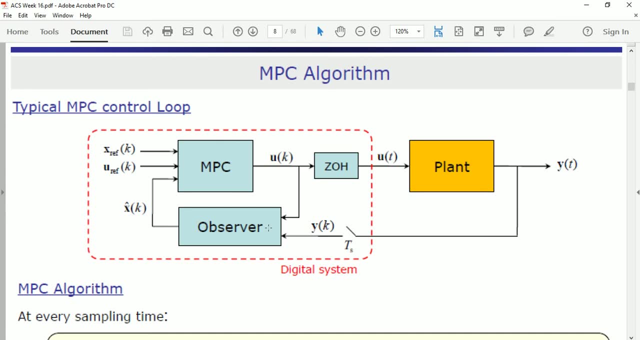 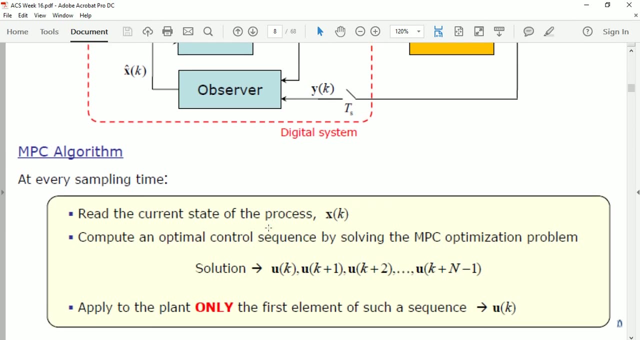 from here. so you are giving it to your MPC and we have already discussed the observer. what are the observer? we have discussed the observer that how it is working. okay. MPC algorithm at every sampling state, read the current state of the process. x of k compute: an optimal control sequence. 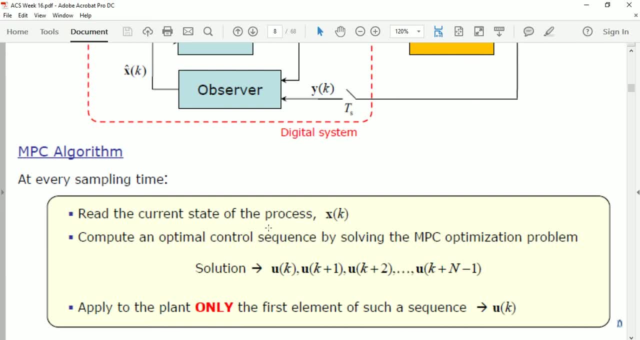 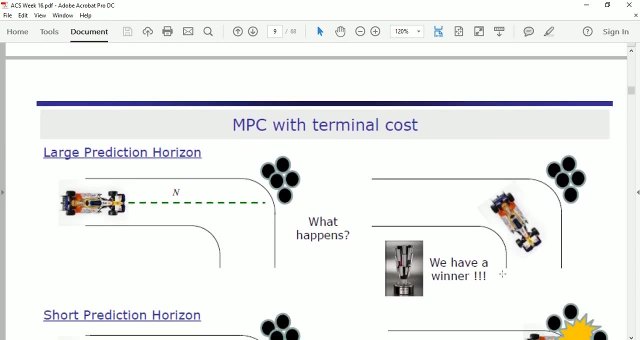 by solving the MPC optimization problem and apply to the plant only the first element of a sequence, that is, u of k. after that it will automatically compute its further values while doing the iteration. okay, MPC, there is one more concept in it: prediction horizon you can see in this: 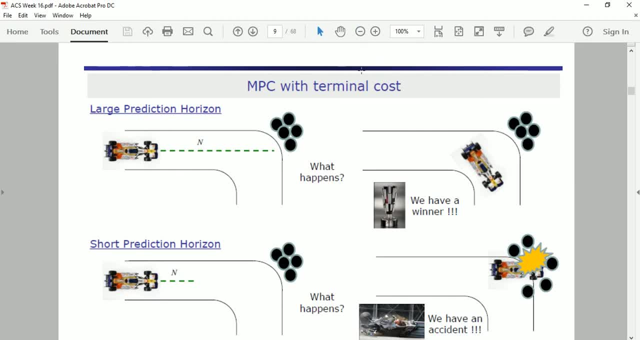 let me zoom out a little. like now: there is a car and there is a MPC in it. if its prediction horizon is very high, if its n is high, then it can safely take turn. otherwise, if your prediction horizon is low and there is a turn coming ahead, 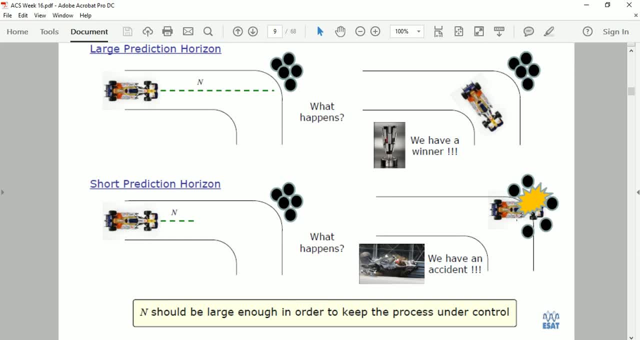 see there is a turn coming in the trajectory, then it can boom, it can, it can hit, so it will be an accident. so the length of the prediction horizon- that is also important that you have to keep it as n, so n should be large enough in order to keep the process under control. 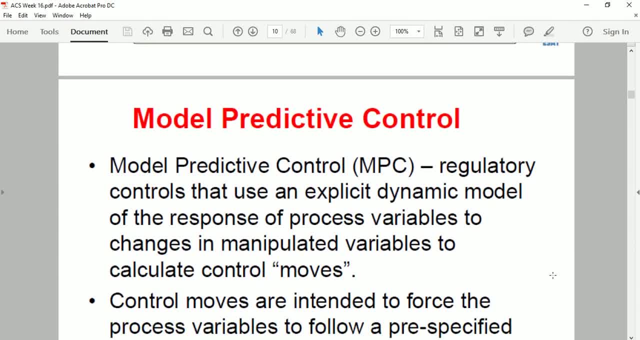 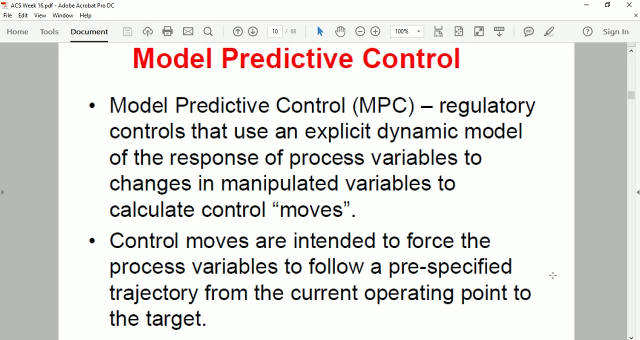 so this is the concept here, basically okay. model predictive control: regulatory controls that use an explicit dynamic model of the response of the process variables to changes in the manipulated variables to calculate control moves. control moves are intended to force the process variable to follow a pre-specified trajectory. 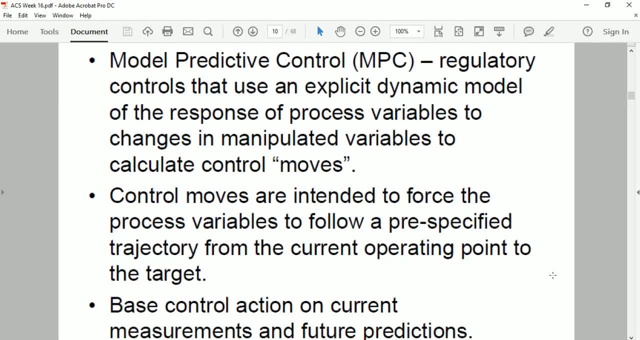 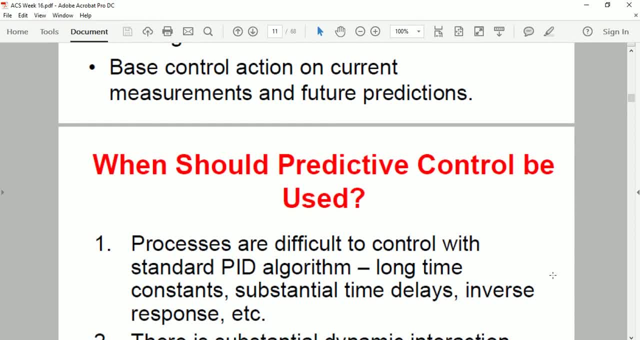 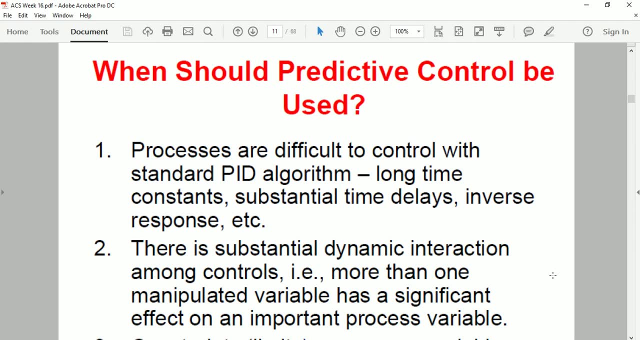 from the current operating point to the target based on control action, on the current measurements and future predictions. future predictions y. so why should predictive control be used? processes are difficult to control with a standard PID control algorithm. long time constraints. long time constraints and delays- substantial time delays. 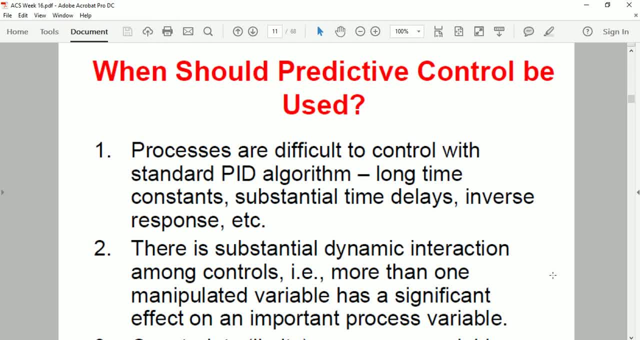 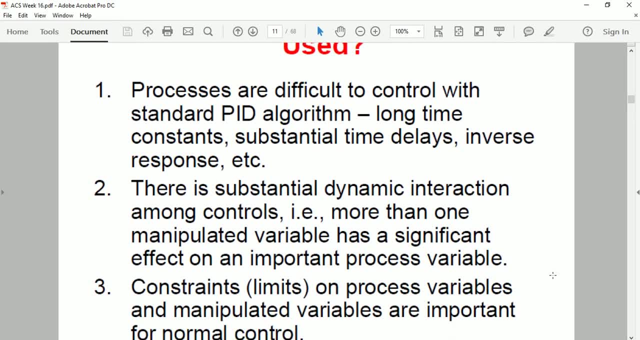 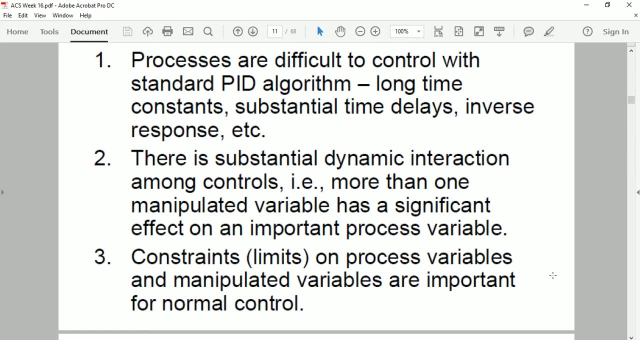 inverse response: higher order dynamics. higher order system PID is not that good for you. there is substantial dynamic interaction among controls that is more than one manipulated variable has a significant effect on the important process. variable constraints and limits on the process. variables and manipulated variables are important for normal control. 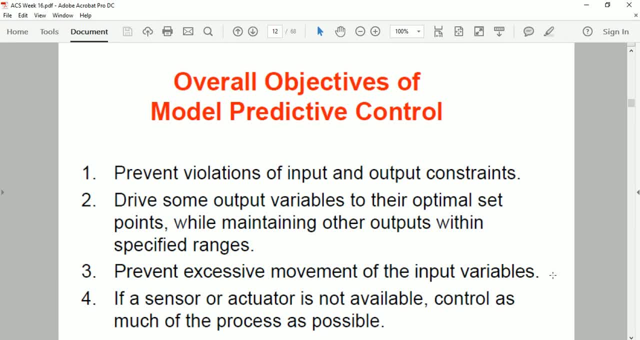 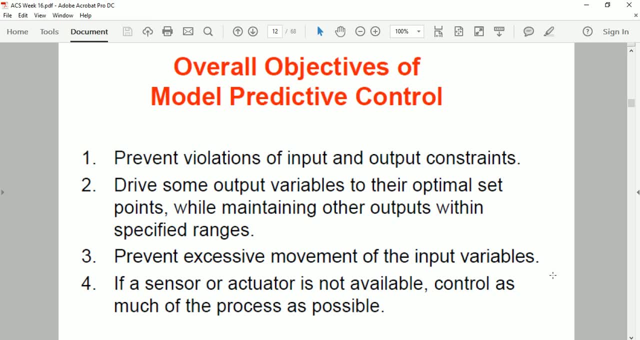 overall objective is model predictive control. prevent the violations of input and output constraints. it will be within the constraints. drive some output variables to their normal optimal set points while maintaining their outputs within specified ranges. prevent excessive movement of the input variables if a sensor or actuator is not available. 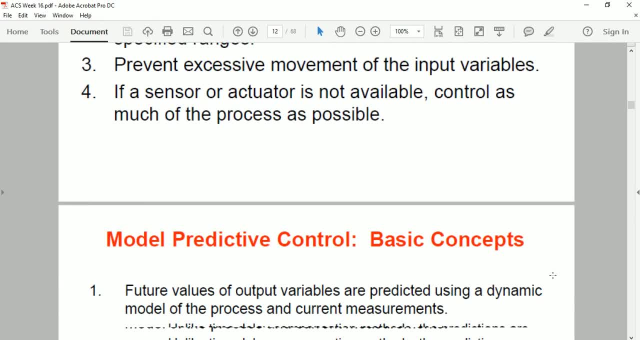 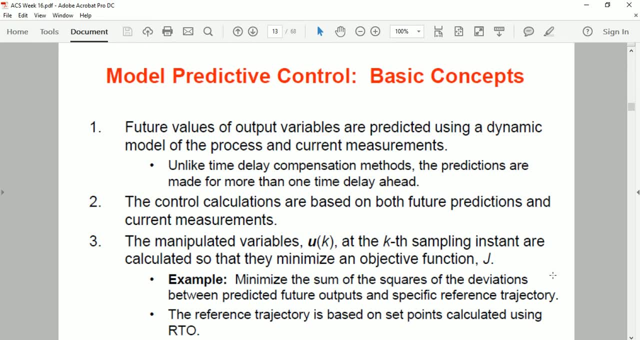 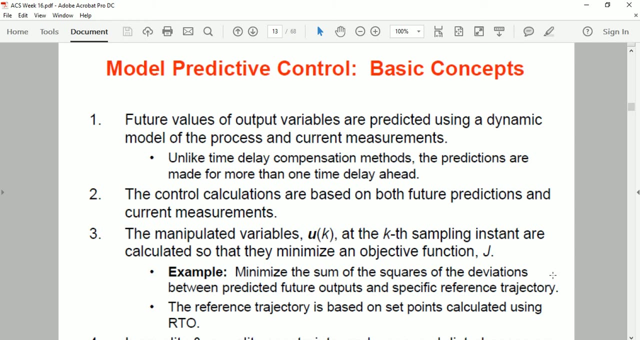 control as much of the process as possible. okay, what are future values? future values: future values of output variables. future values of the output variables are predicted using a dynamic model of the process and current measurements. unlike time delay compensation methods, the predictions are made for more than one time delay ahead. 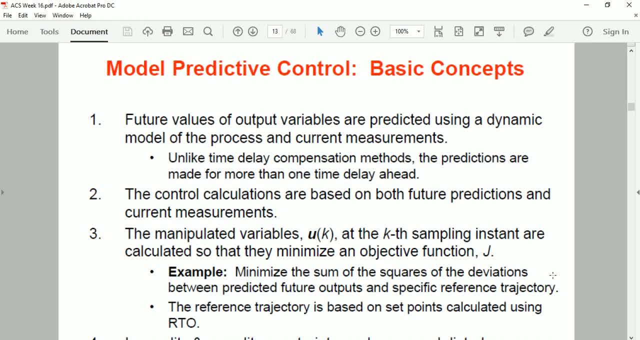 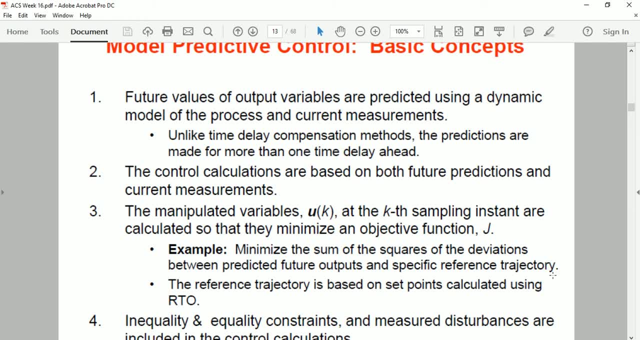 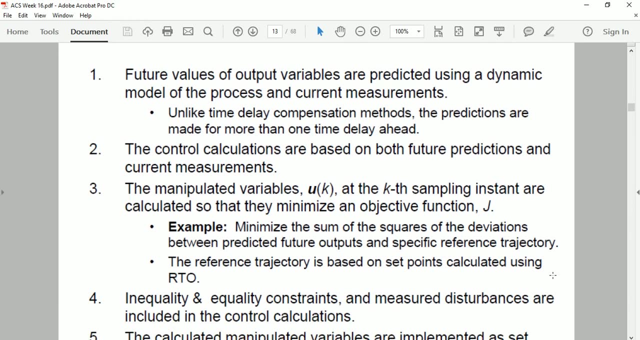 the control calculations are based on both future predictions and current measurements. the manipulated variables u at the k-th sampling instant are calculated so that they minimize an objective function. j minimize the sum of squares of the deviations between predicted future outputs and specified reference trajectory. the reference trajectory is based on the set points. calculating using RTO. 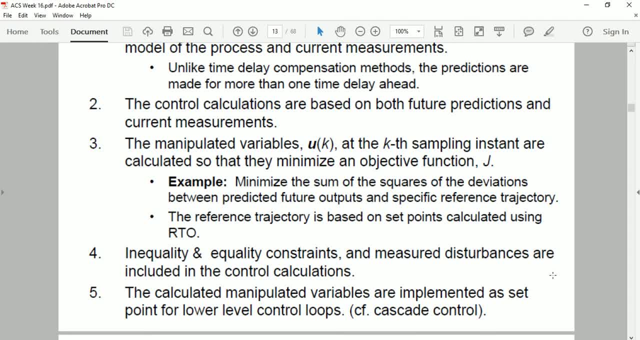 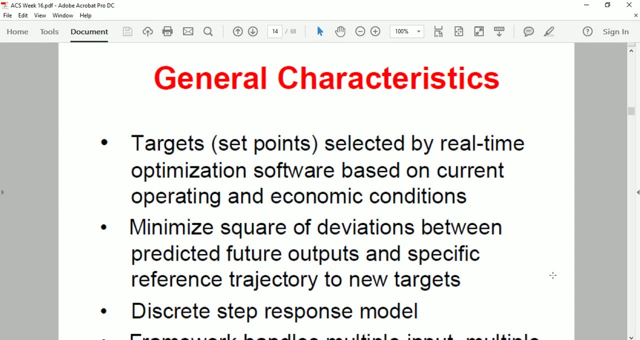 okay. inequality or inequality constraints and major disturbances are included in the control calculations. the control manipulated variables are implemented as set points for the lower level control loops. what are the general characteristics, targets or set points selected by real-time optimization software based on the current operating energy economic conditions? 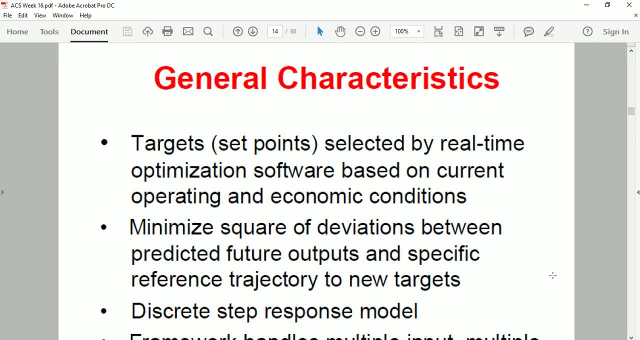 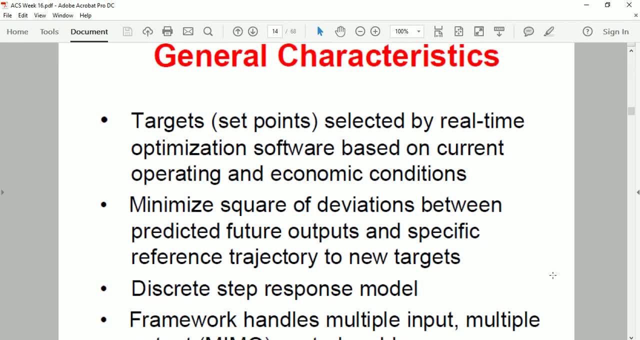 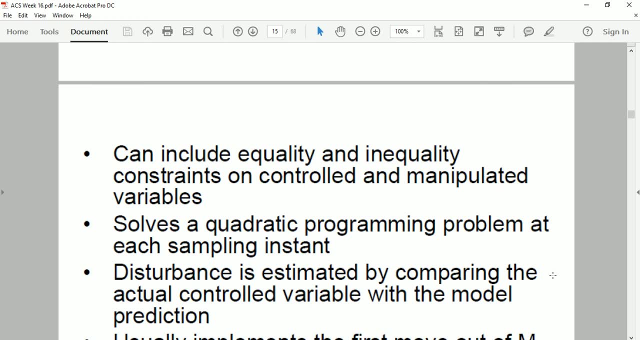 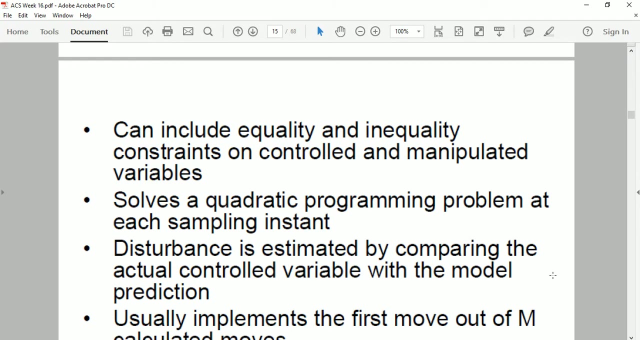 minimize the scale of deviations between the predicted future outputs and specified reference trajectory to the new targets. discrete step response model framework. handles multi-input and multi-output control problems. can include equality and inequality. constraints on controlled and manipulated variables. solves a quadratic programming problem at each sampling instant. 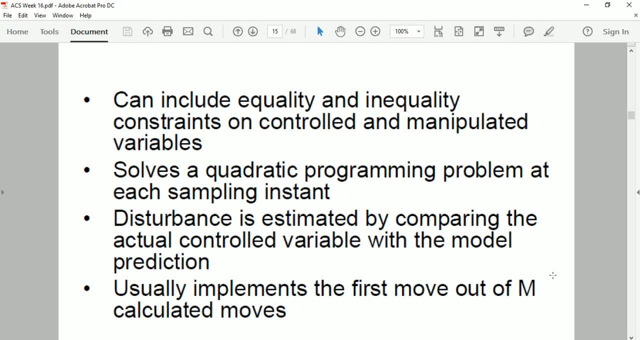 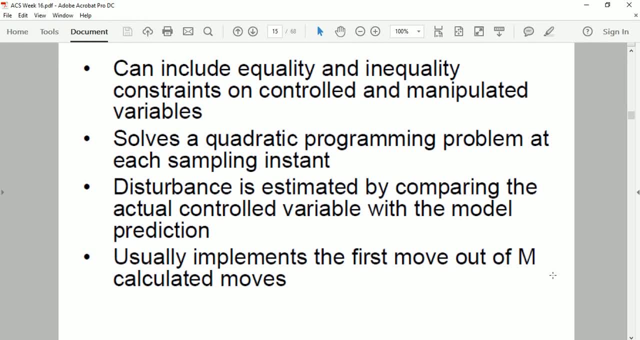 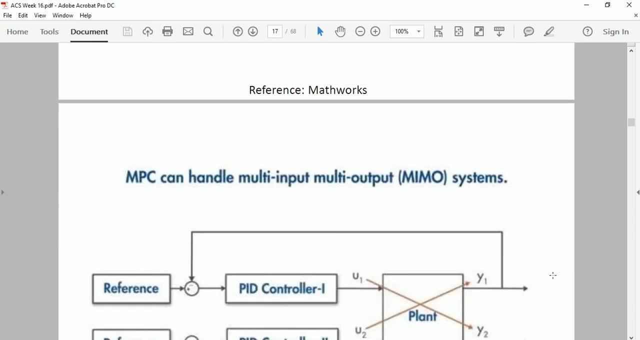 disturbances determines, is estimated by comparing the actual model variable with the model. prediction usually implements the first move out of capital: M calculated moves. okay, the same thing is repeated again and again. okay, MPC can handle multi-input, multi-output systems. okay, okay, MPC can handle multi-input, multi-output systems. 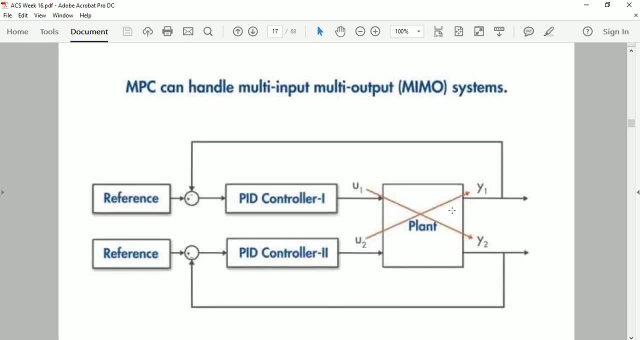 as you can see here, if you have multi-input, multi-output systems, okay, then MIMO system in which y1 depends on y1, u1 and u2 and y2 depends on u1 and u2. so what you do is this PID controller which you have. 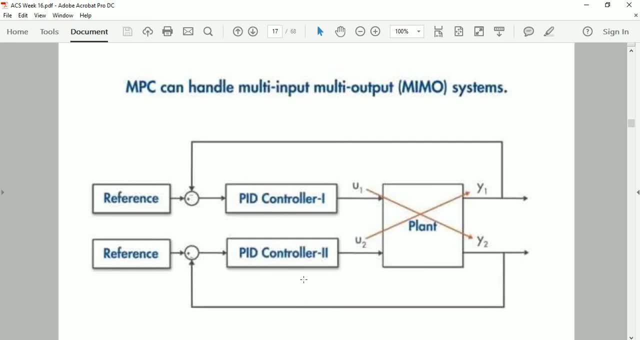 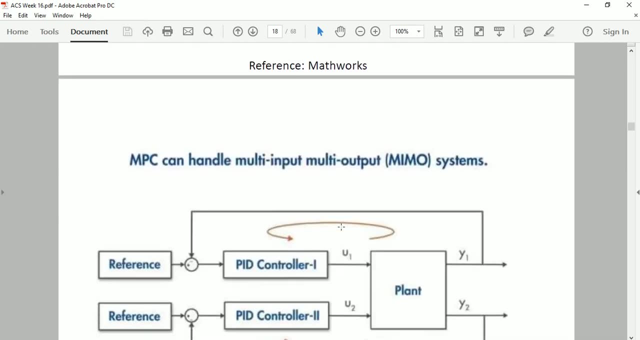 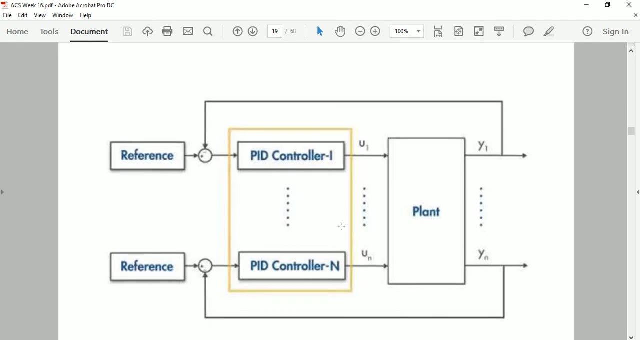 for this loop, for this loop, but there is interaction. then what will you do here? for MIMO system? you will use MPC here. MPC can handle multi-inputs and multi-output systems. okay, now look inside this. what will you do? by combining all of them, by combining them. 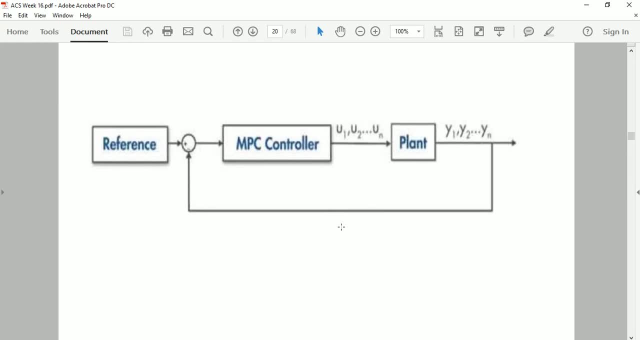 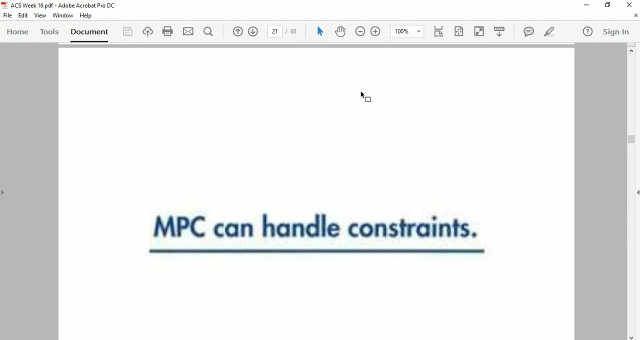 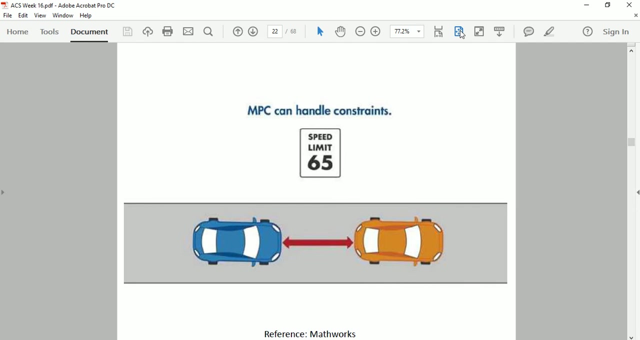 you will put a MPC controller, okay, so MPC can handle the constraints. that means you can take your process to the limits and work with it. you can take it to the limits and work with it and it can handle the constraints. like now: you have a car. it has to maintain this distance. 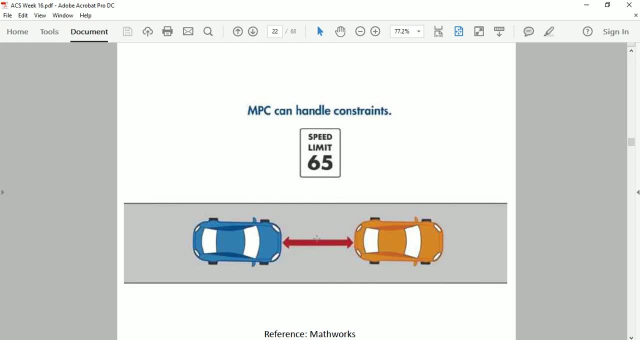 okay, you have to work with it and maintain this distance. this will be the constraint. so because of this constraint, you can say that MPC will be beneficial for you. there is no such thing in a PID controller. and okay, and apart from this, MPC has preview capability. that means it can anticipate the future. 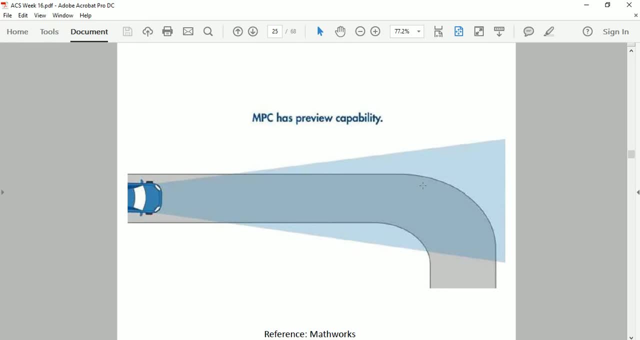 look inside this, as there was an observer inside it so it can preview. it has a preview capability, okay, and if there is a preview capability, then look here, if your car is going and there is MPC installed in it, so if there is a preview capability in it. 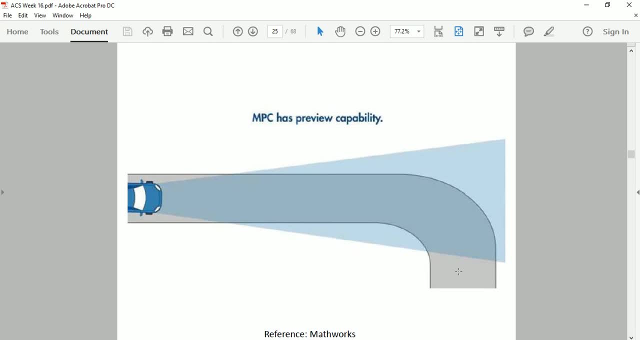 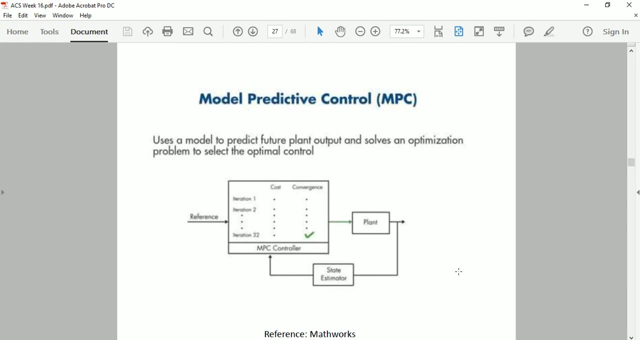 then it can take turn. when it will reach here, then it can take turn. okay, if it is not there, then it can collide, okay. model predictive control uses a model to predict future plant. model predictive control- it is also mentioned in the name. predictive control uses a model to predict. 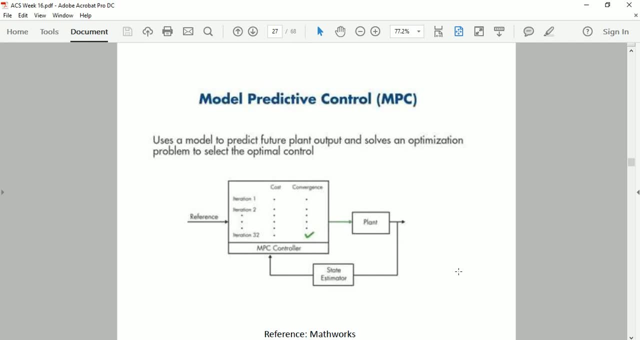 the future plant output and solves an optimization problem to select the optimal control, like here, there is a state estimator in which the algorithm of MPC is running, in which the value will go from here and your J function will be calculated. it will be minimized cost function. we have already discussed 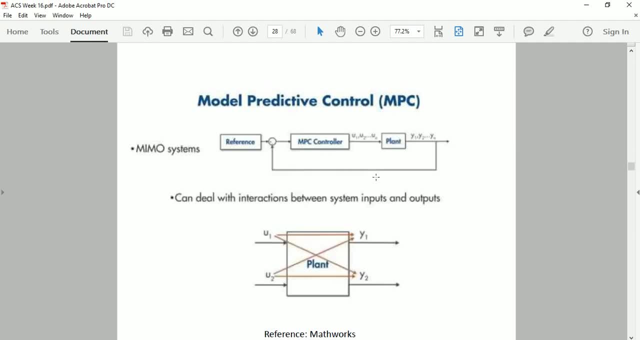 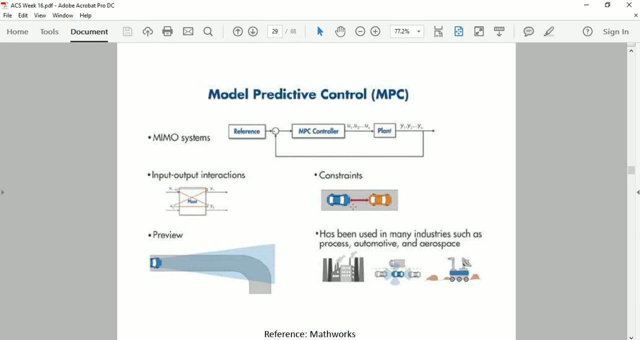 this kind of diagram earlier. okay, so what is in MPC controller for MIMO systems? it can handle the interactions between inputs and outputs. okay, it has the ability of preview. it has been. it can be with respect to constraints. okay, it has the ability of preview with respect to constraints. 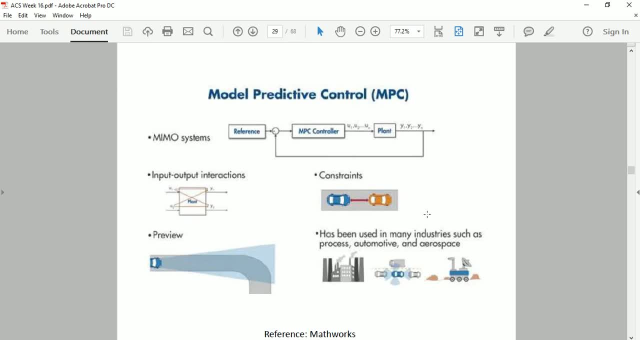 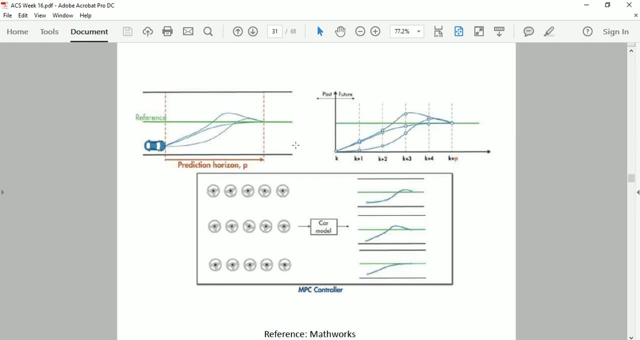 it has been used in many industries, such as process, automotive and aerospace. and okay, now, like this is an example in which you have a car, it is, it is at time t and this is at time t plus capital t. now it has you see in prediction horizon. 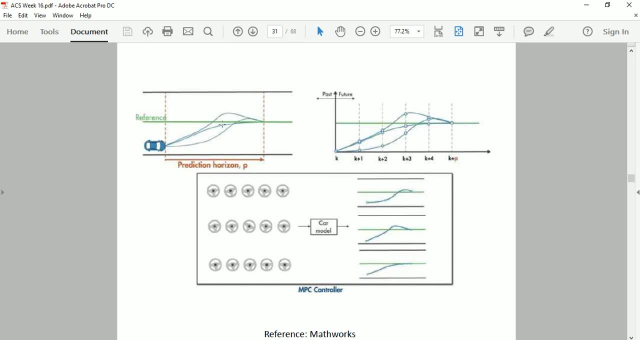 it has various paths. it has which it can follow, which it is getting from its estimator. now it has to select which will be optimized from these three so that the cost function will be minimum, like now. this path is coming. this path is coming. this path is coming. 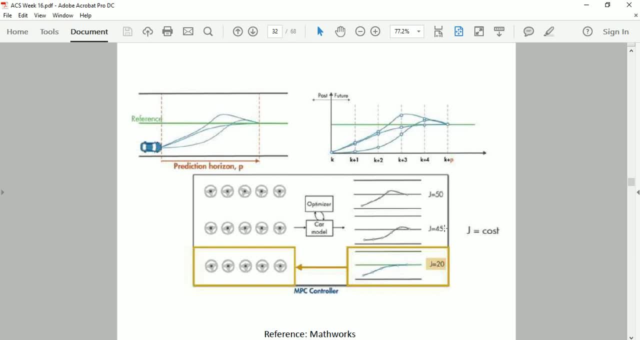 okay, now what will the car do? the car on which the cost function will come out 50,, 45,, 20. see, your cost is the lowest on 20, so the car will follow this path, which that is the beauty of the model: predictive control. 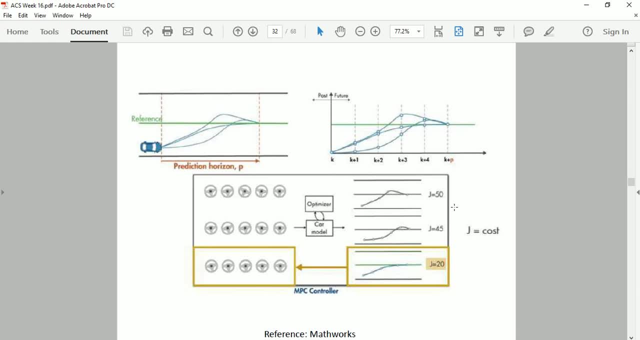 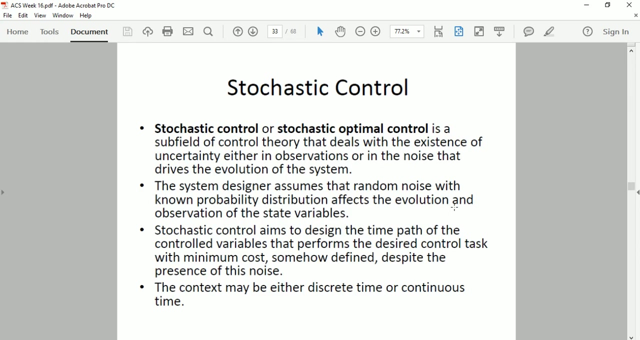 see how many things have come in it in this prediction. MIMO system has come in this prediction, so this is a very powerful controller where your system, if higher order systems come and MIMO systems come and there are time delays, so there you consider MPC, okay, next. 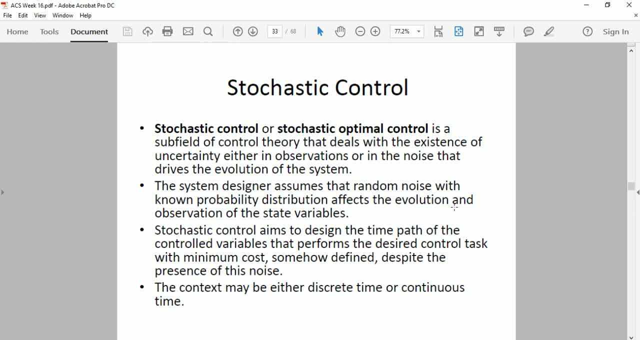 our topic is, after MPC, stochastic control, what is stochastic control? stochastic control, stochastic control and stochastic optimal control- is a subfield of control theory that determines the existence of uncertainty, either in observations or in the noise that drives the evolution of the system. the system designer assumes that. 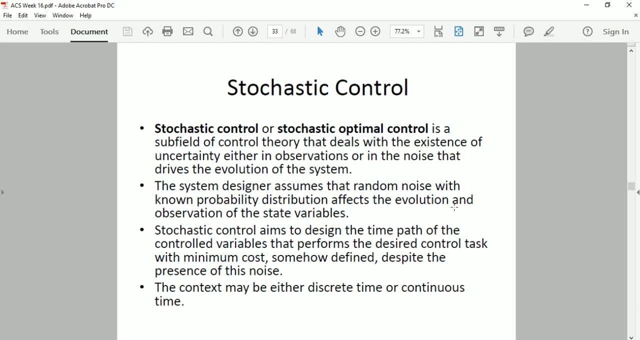 random noise with known probability distribution affects the evolution and observation of the state variables. stochastic control aims to design aims aims to design the time path. aims to design the time path means minimum cost somehow defined despite the presence of the noise. stochastic control is opposite of deterministic control. 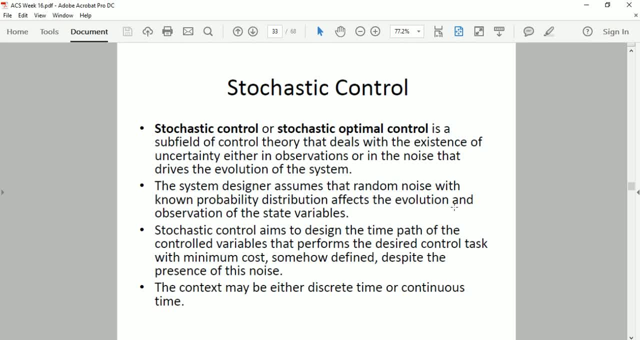 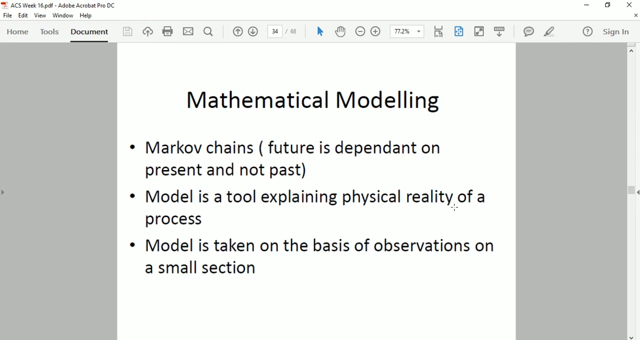 deterministic control is the equation, the input and output. the stochastic control is the stochastic processes which are stochastic, which are random, any stochastic. you have these stochastic functions that you can just estimate it now in mathematical modeling. mark of change. mark of change is future, is dependent on the present and not past. 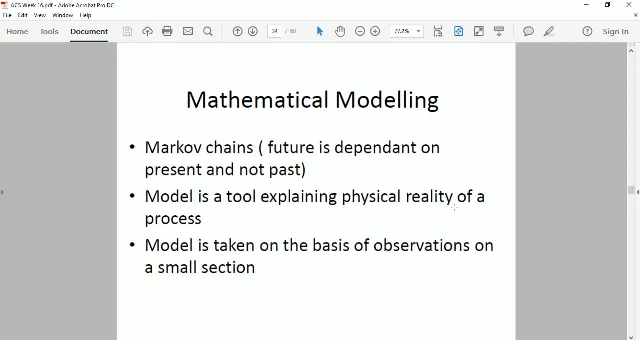 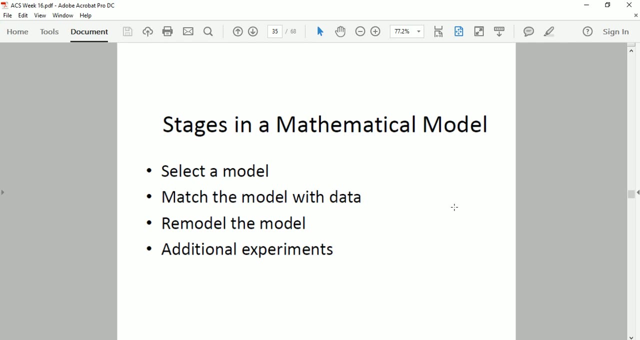 future is dependent on the present and not past. model is a tool explaining physical reality of a process. model is taken on the basis of observations, on a small selection. what are the stages in mathematical modeling? we select a model, match the model with the data, remodel the model. 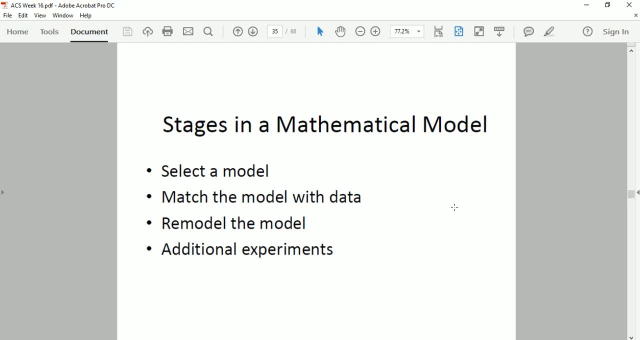 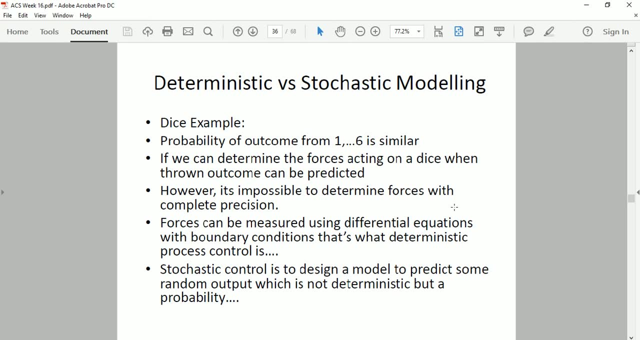 and do additional experiments so that the error ends. so we do modeling like this. so in deterministic vs stochastic modeling, like you have dice problem, like you have 6, there is possibility. probability of the outcome from 1 to 6 is similar if we can determine the forces acting on a dice. 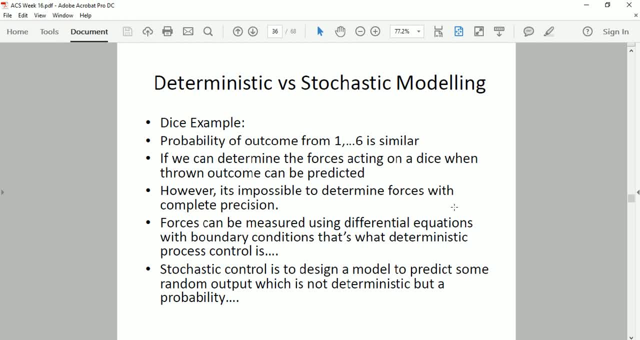 it can be predicted. however, it is impossible to determine forces with complete precision. forces can be like you have dice: you are not sure what will come. you can predict it. what is the probability of 1,, 2, 3? so probabilistic is your process and stochastic control. 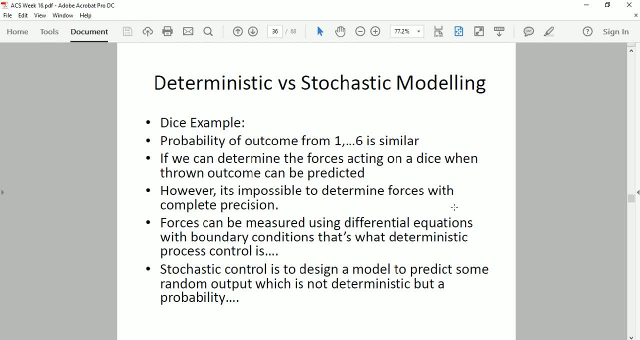 is your probabilistic control system. however, it is impossible to determine the forces with complete precision. forces can be measured by differential equations with the boundary conditions. that's what deterministic process control is. stochastic control is to design to predict some random output which is not deterministic but a probability. 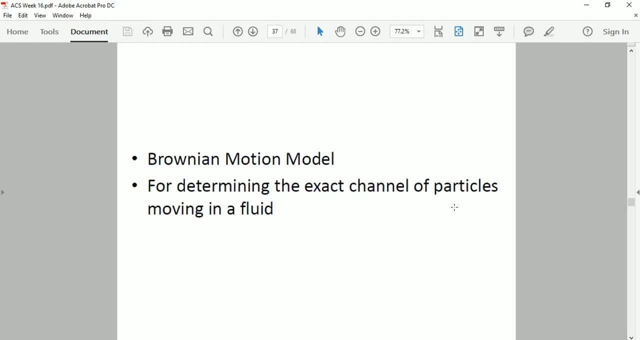 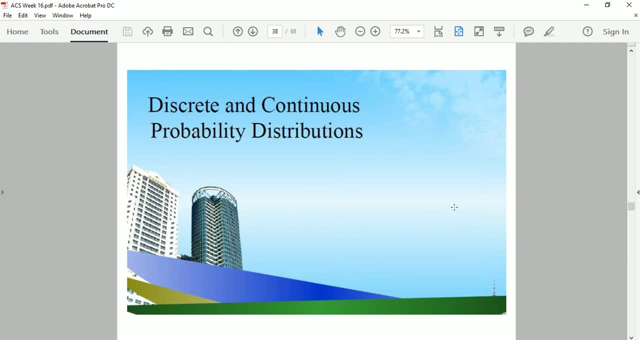 which I have discussed with you. Brownian motion model is for determining the exact channel of particles moving in a fluid. now in stochastic control, the distributions related to stochastic are very important. we should have knowledge of it. discrete and probability distributions are of two types: discrete and continuous. 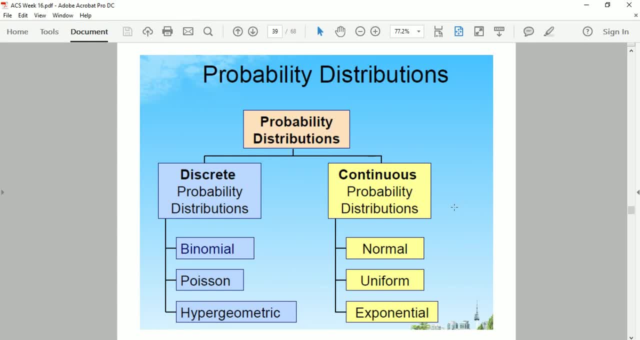 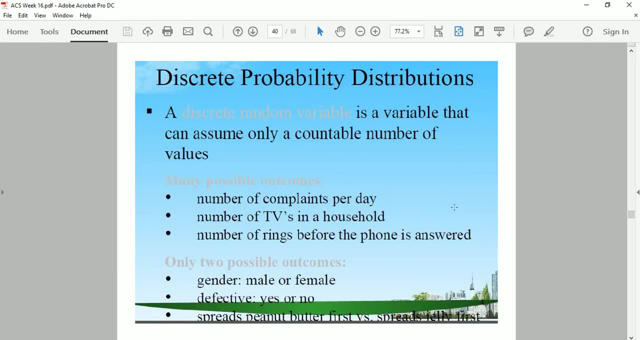 in discrete probability distributions. binomial comes, Poisson comes, hypergeometric comes and continuous has normal, uniform and exponential. what will be discrete probability distribution? discrete random variable is a variable that can assume only accountable number of values. discrete means any value of this finite value. 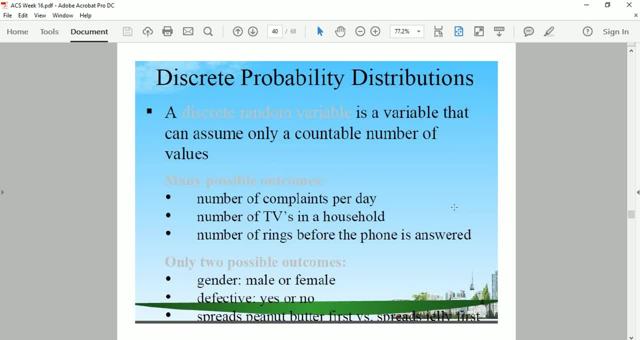 for example: many possible outcomes: number of complaints per day, number of TVs in a household, number of rings before the phone is answered. only two possible outcomes are discrete. only two possible outcomes are: binary gender, male or female. defective: yes, no, spread minute buffer first. 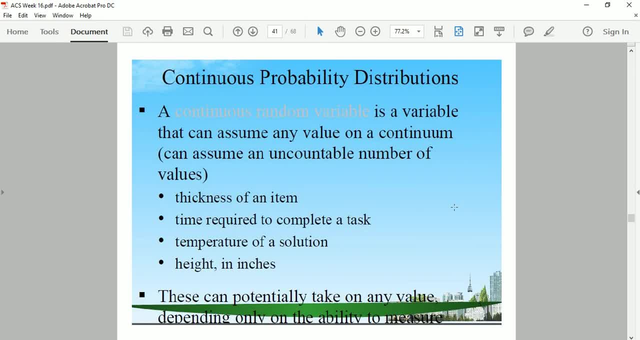 versus spreads jelly. first, what is a continuous random variable? it is a variable that can assume any value on a continuum, like a continuous number, like you have a real number between 0 to 1, it can have any value. it can have any value between 0 to 1. 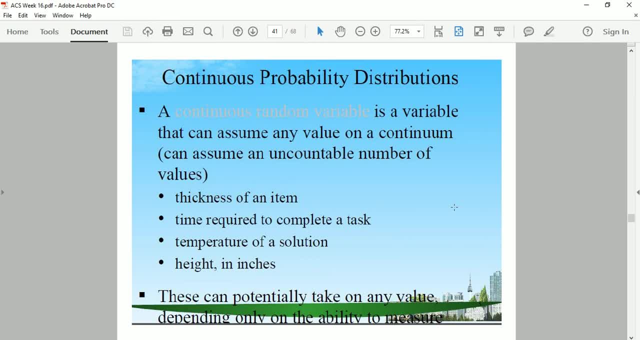 0.99999. it can assume any value on a continuum in a specific set. can assume any uncountable number of values like thickness of an item, time required to complete a task, temperature of a solution. height in inches. you can go further in decimal places. 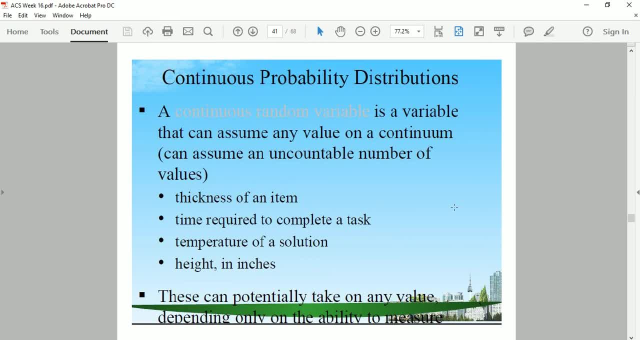 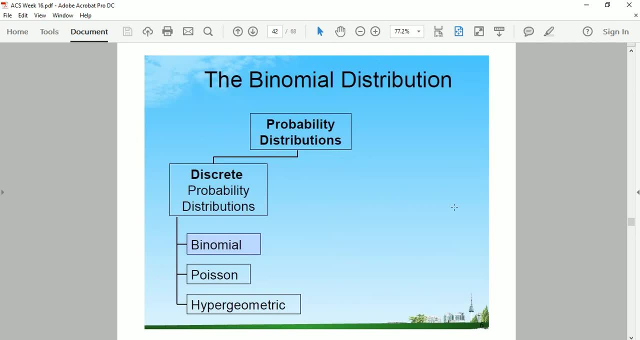 there is no limit. these can potentially take on any value, depending on the ability to measure. how much can you measure it? any value can be obtained. what will be binomial distributions? it comes in discrete probability distributions, in probability distributions, discrete volume, binomial Poisson and hypergeometric binomial. 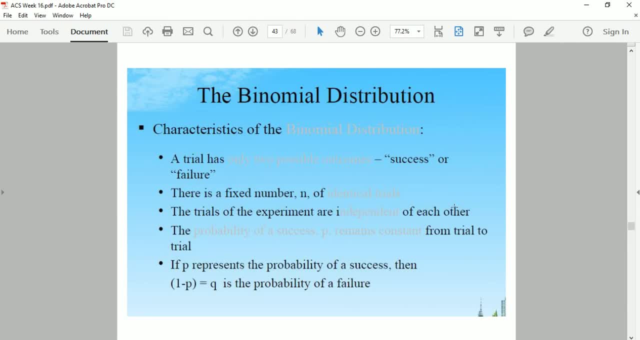 what are the characteristics of the binomial? a trial has only two possible outcomes: success or failure. success or failure. a trial has two possible outcomes. there is a fixed number n of the identical trials. the trials of the experiment are independent of each other. the probability of success. 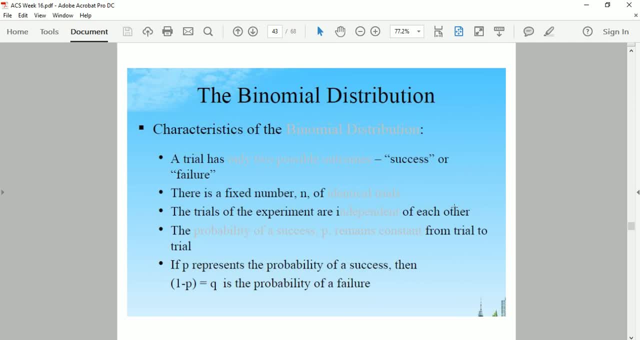 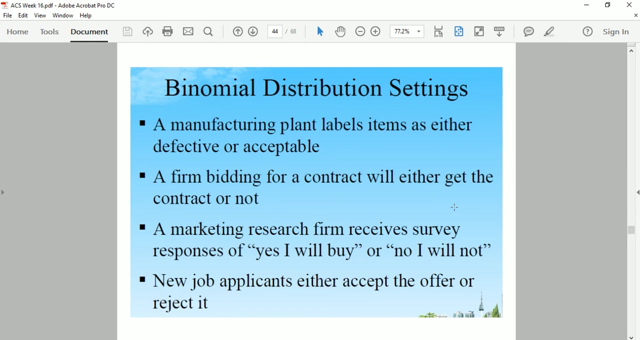 P remains constant from trial to trial. if P represents the probability of success, then 1-P is the probability of failure. if P is success, then 1-P is the probability of failure. how will we do binomial distribution? setting a manufacturing plant labels items as either defective or acceptable? 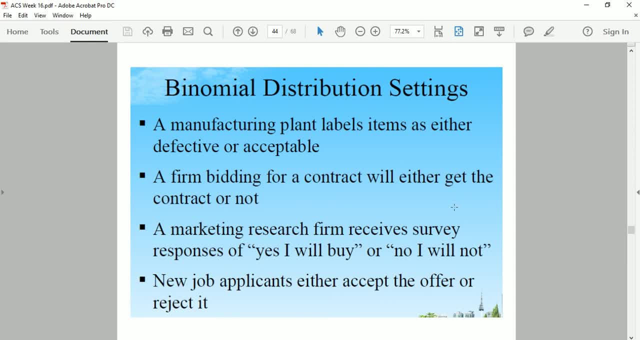 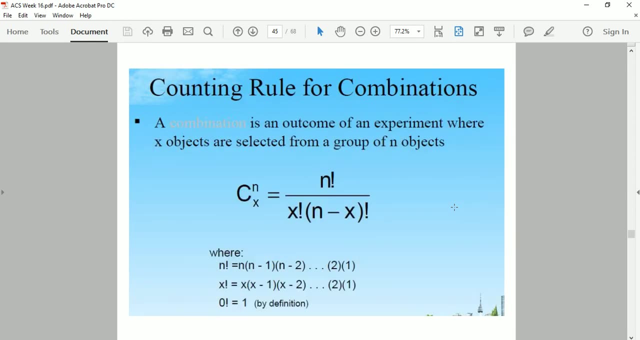 a firm binding for a contract will either get the contract or not. market research firm receive survey responses of yes I will buy or no I will buy. there will be two outcomes: new job applicants either accept the offer or reject it. combination combination is used. combination is an outcome of an experiment. 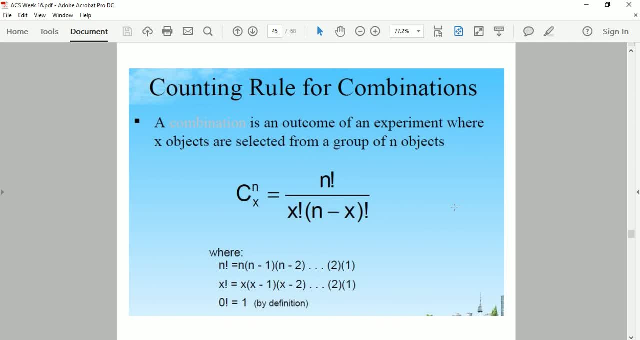 where the x objects are selected from a group of n objects. combination does not matter. cnx is equal to n. factorial over x. factorial into n minus x factorial, n factorial is n into n. factorial, n minus 1, n minus 2, so on up to 2 into 1. 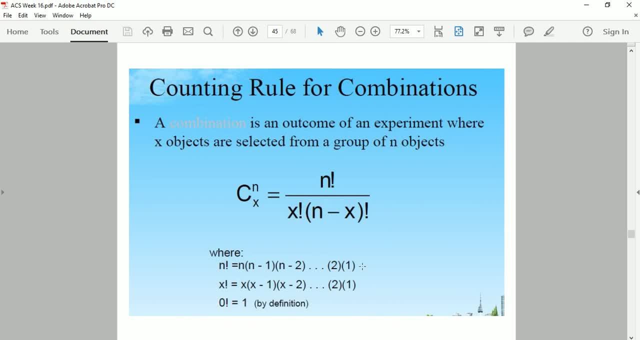 these are the products. so this is the basic in your BS probability course. what is the combination of these things? what is your permutation permutation combination: what is x factorial, x into x minus 1, x minus 2 into, so on? what will be 0 factorial? it is 1. 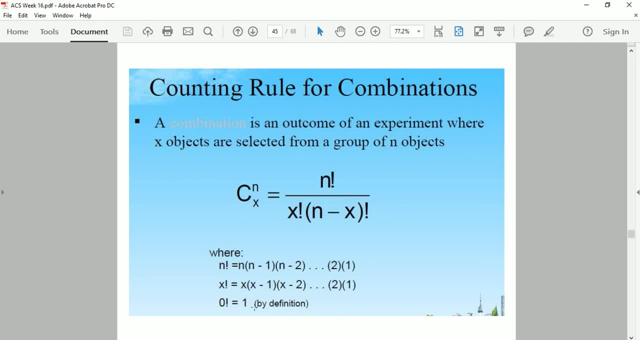 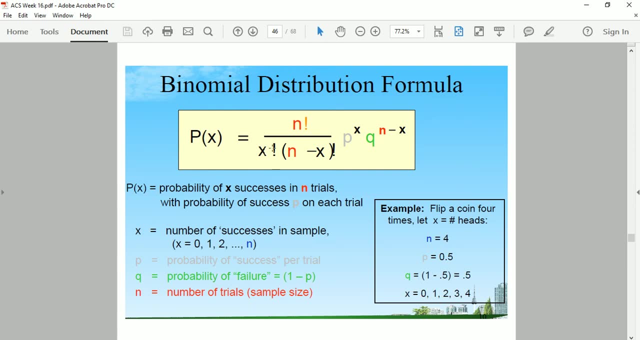 basically, this is 0 factorial, that is 1. ok, and see, this permutation came that is n factorial over x factorial. ok, this permutation in this basically combination, this combination is being used here and that is your probability of x. this is the binomial distribution formula, that is, p of x is equal to. 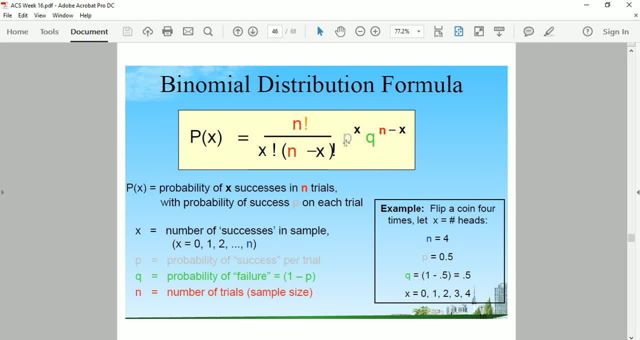 n factorial over x factorial into n minus x. factorial power of p is x. power of q is n minus x. ok, what is x random variable here? p of x is probability of x successes in n trials. means in n trials, x success with probability of success p. 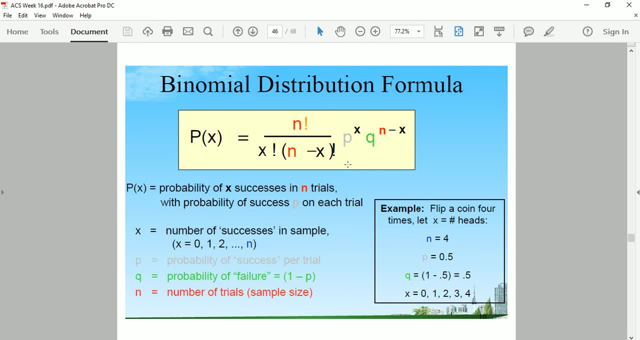 on each trial and in each trial the probability is p. what is x? number of successes in sample: 0, 1, 2 up to n? p is the probability of success per trial, q is the probability of failure, n is the number of trials. so in example, 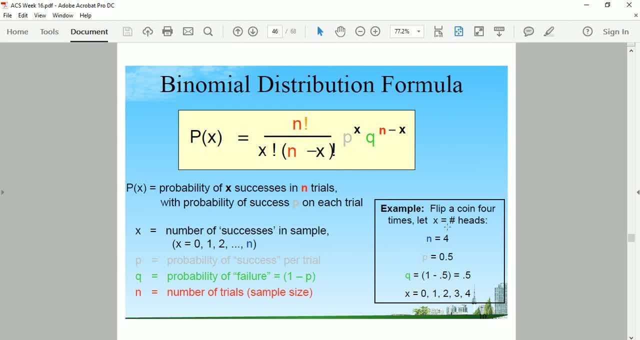 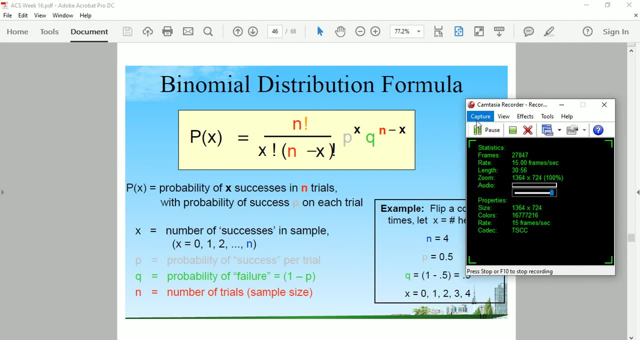 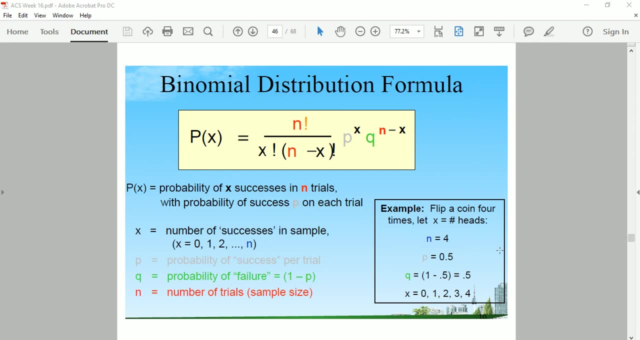 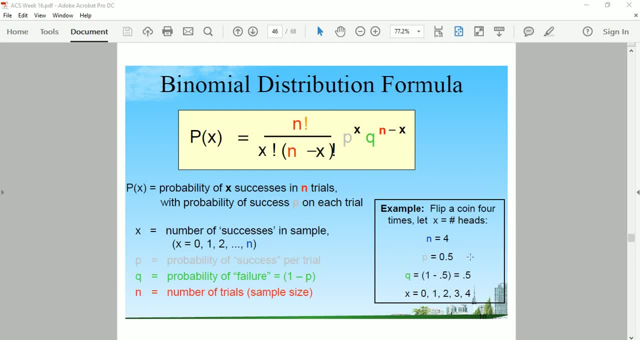 n is equal to 4 and each one has the probability of 50% if it is a fair coin. so if it is 50%, so p equal to 0.5. what does q bring? 1 minus 0.5, that is 0.5. 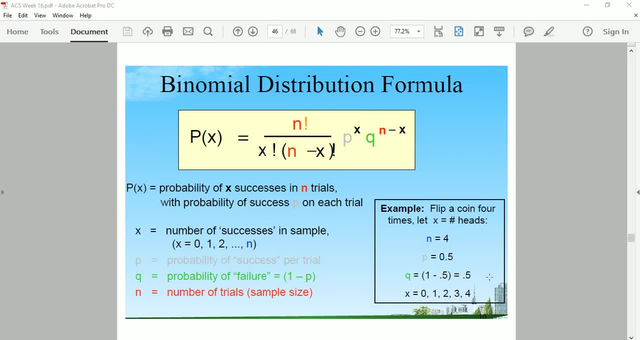 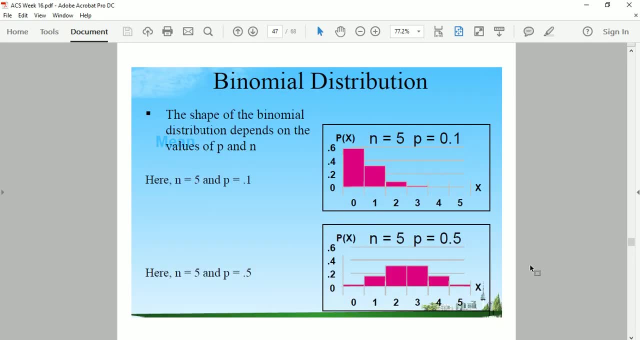 and what does x bring? 0, 1, 2, 3, 4. ok, now in this binomial distribution here for this, the distribution is the shape of binomial distribution, depends on the values of p and n. so now you can see that the distribution of p and n depends on the shape of binomial distribution. 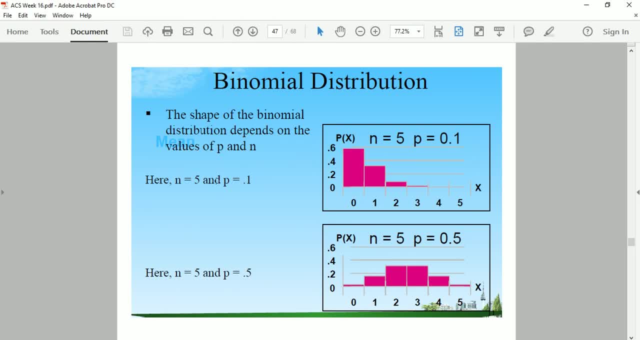 for example, if your probability of success is 5 and your probability of success is 0.1, then you can see that if there is no success in 0,, then your probability is higher. if there is no success in 0,, then your probability is lower. 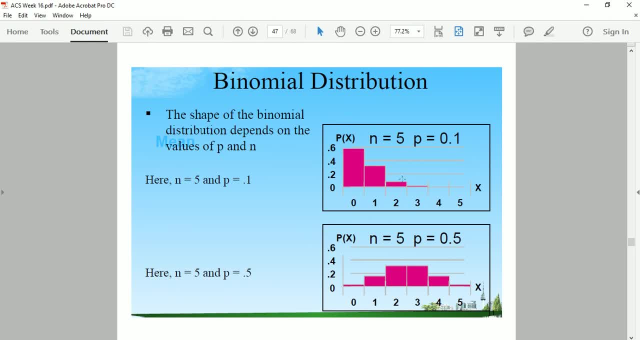 so in this case you can see that the distribution of p and n is downward. in the second case, you can see that the distribution of n is 5 and your probability is 0.5. so your binomial distribution is like this. so the distribution of p and n depends on the value of p. 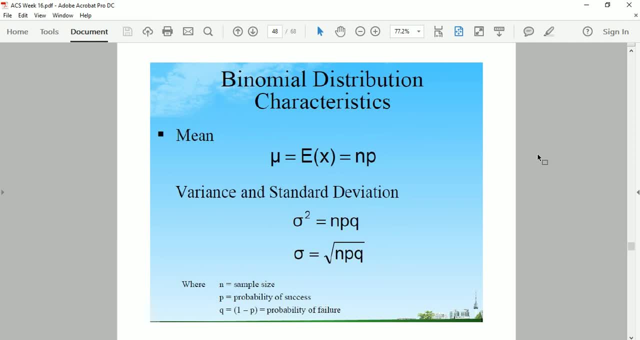 and n depends on the value of p and n. so the distribution of p and n depends on the value of p and n. now let's see the characteristics of binomial distribution. mean is equal to e of x, that is, n, p and variance and standard deviation. 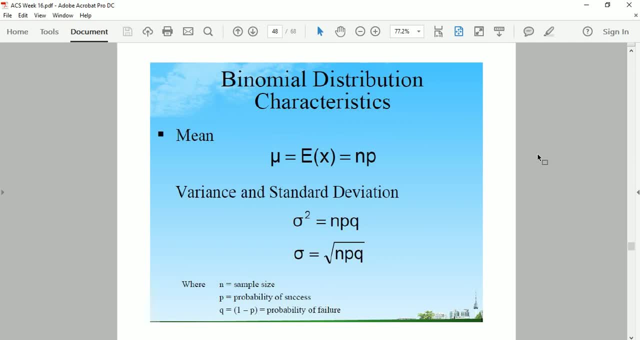 mean value and standard deviation are two important parameters. mean value is expected value, that is n- p, and variance is n p q. sigma is your standard deviation. sigma is equal to under root. n p q. sigma is your sample size. p is your probability of success, n q is the probability of failure. 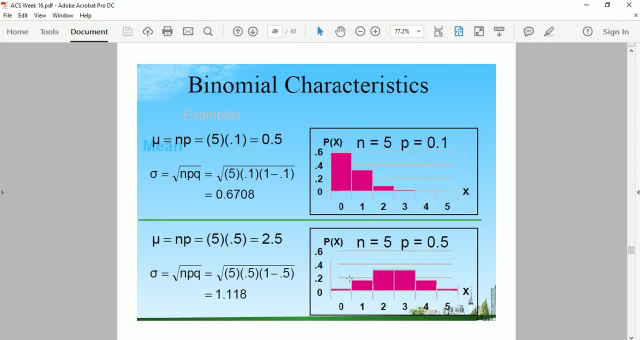 now let's apply the binomial characteristics. for example, what will be the mu of this distribution? in this case, mu will be n, p, n is equal to 5 and p is equal to 0.1. that is 0.5. mu is your 0.5. 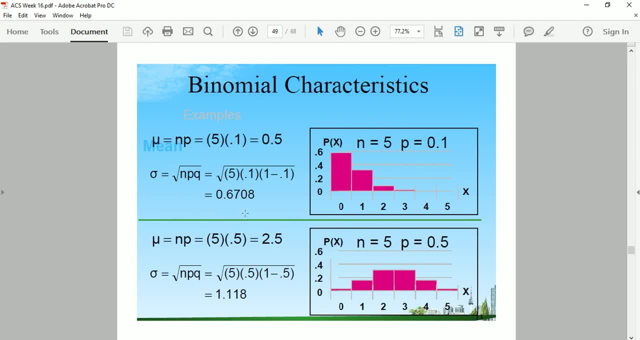 and sigma will be n p q, that will be 0.6708, and for the lower distribution, mu will be 2.5 and n p will be 0.5 and sigma will be n p q, that is, 1.118. so this was a simple example. 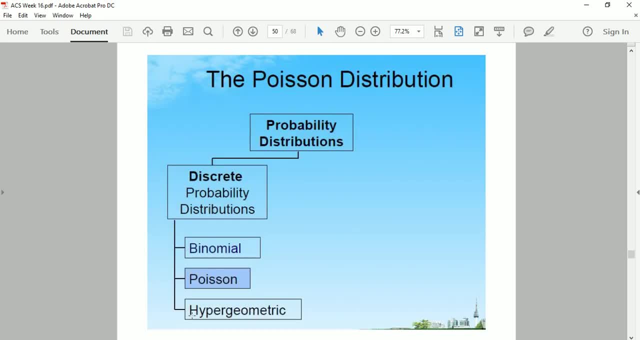 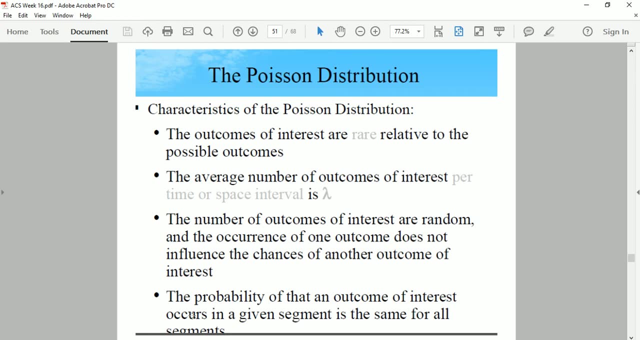 to demonstrate its calculations. next, let's discuss Poisson, the characteristics of the Poisson distribution. the outcomes of interest are rare relative to the possible outcomes. the average number of outcomes of interest per time or space is lambda. this is the average number of outcomes. the number of outcomes of interest are random. 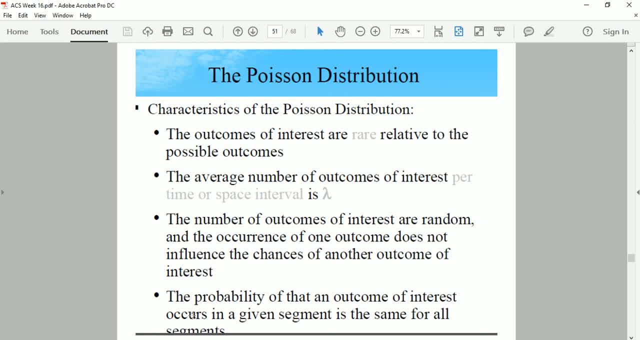 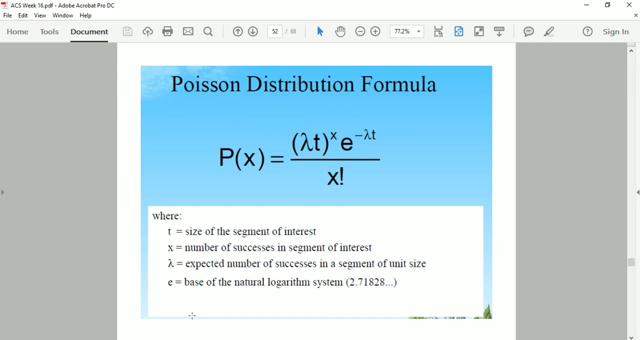 and the occurrence of one outcome does not influence the chances of another outcome of interest. it is independent. the probability of that an outcome of interest occurs in a given segment is the same for all the segments. so this is the Poisson formula. p is equal to lambda t. 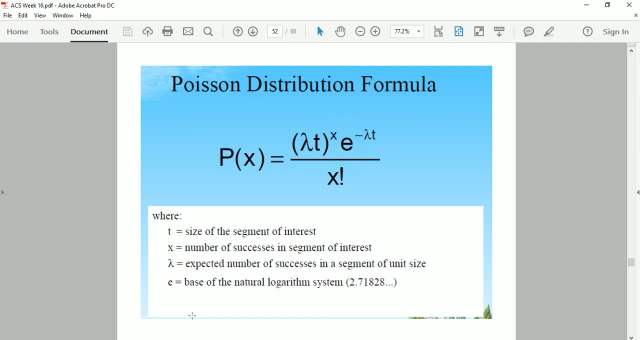 power x, e raised to the power minus lambda t over x. factorial. now, t is the size of segment of interest, x is the probability of successes and segment of interest lambda is the expected number of successes in a segment of unit size. e is the base of the natural logarithm. 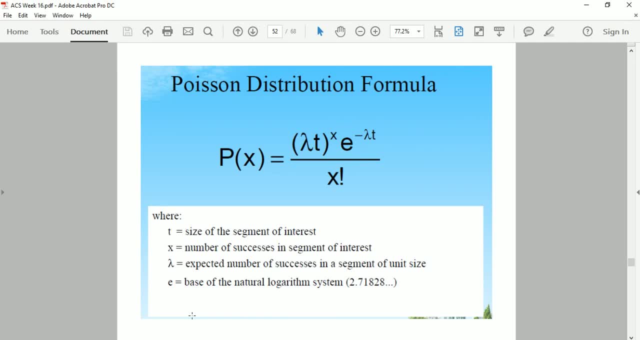 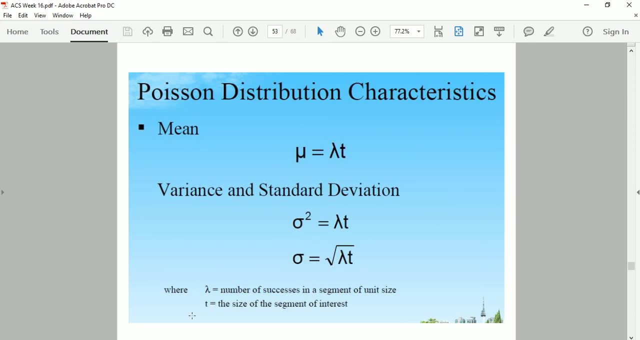 2.71828. the mean of this is: mu is equal to lambda t and its standard deviation and variance is sigma. square is equal to lambda t. sigma is equal to, under root, lambda t. lambda is the number of successes in a segment of unit size. now let us move. 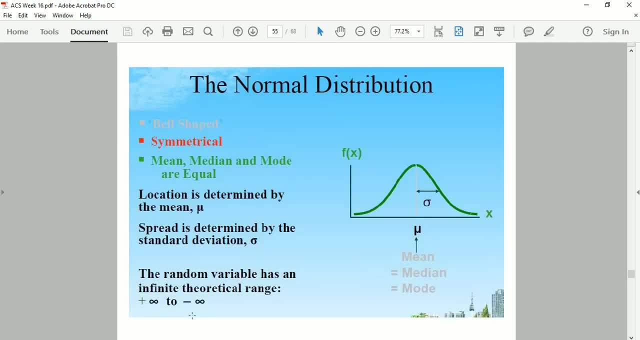 towards normal distribution data. once, when there is normal distribution, it is called bell curve. this is bell curve. it is symmetrical and mean and mean equal to the median. if you calculate average value median. that is the calibrated data set crowd. is the median mod something on a data set? 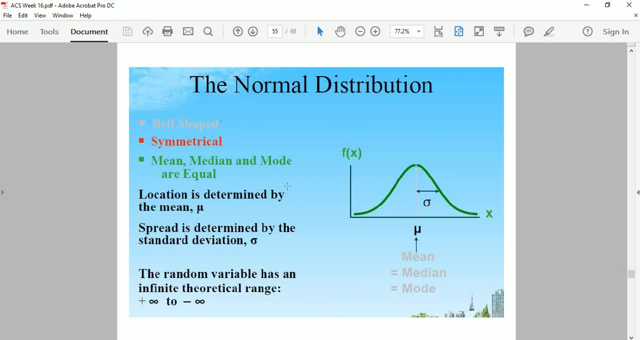 This is known as MOD. This is the knowledge of statistics. location is determined by their mean. spread is determined. this is also called spread. spread is determined by the standard deviation sigma. the random variables has an infinite theoretical horizon, from minus infinity to plus infinity to minus infinity. Now, 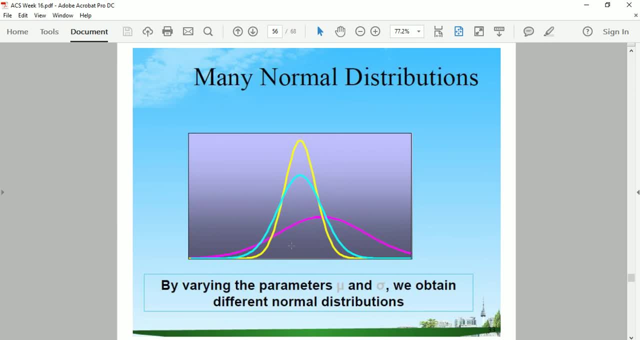 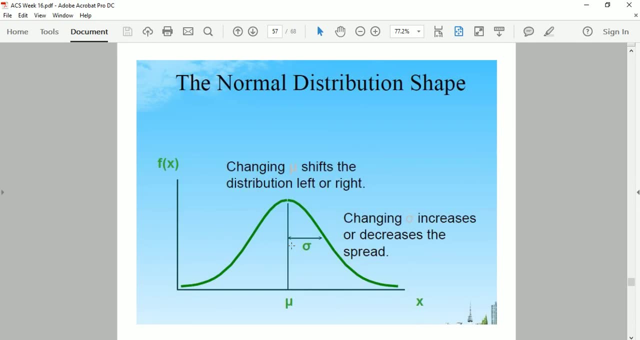 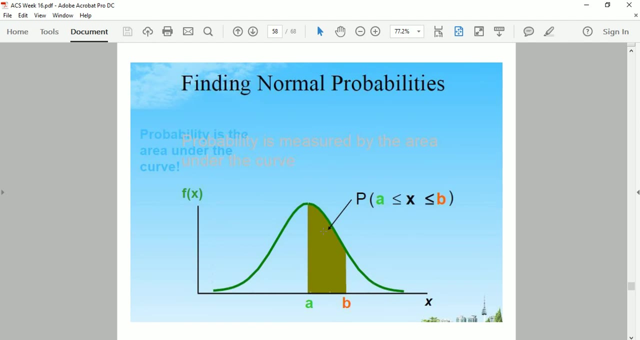 by varying the parameters mu and sigma we obtain different normal distributions. changing the mu shifts the distribution left to right. changing the sigma increases or decreases the spread. Now probability is measured by the area under the curve. you have to find the probability of x from a to b. 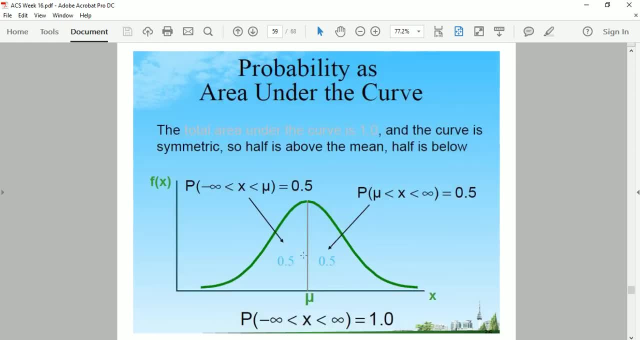 so you have to find the area, and if mu is up to minus infinity to mu is 0.5 to plus infinity to 0.5, then overall the probability of this curve will be 1. the total area under the curve is 1 and the curve is symmetric. 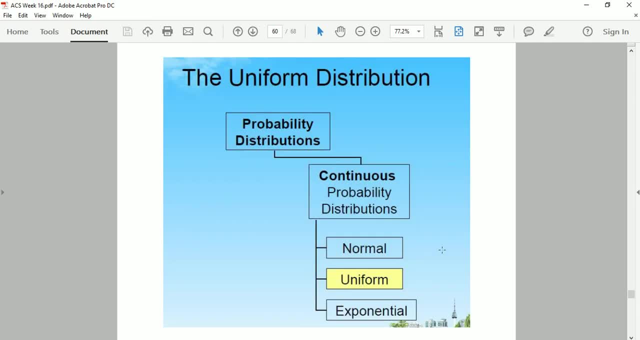 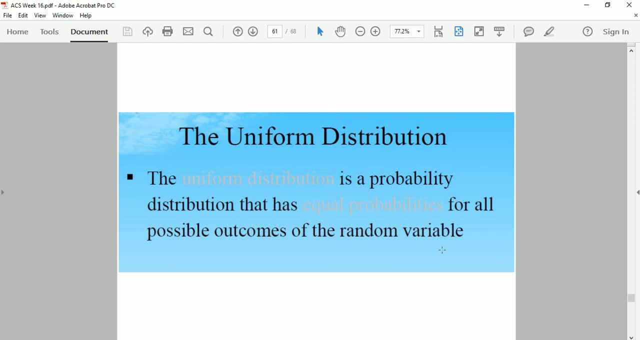 so that half is above the mean and half is below. The next popular distribution is the uniform distribution. Uniform distribution is a probability distribution that has equal probabilities for all possible outcomes and variables. The formula for this is: The continuous uniform distribution is 1 over b minus a. 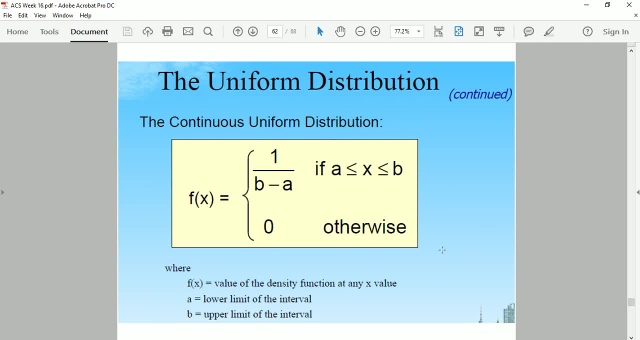 if x is a to b, ie greater than a, greater than equal to a and less than equal to b and f. that is the value of density function. ie value of x. a is the lower limit and b is the upper limit, as you can see, 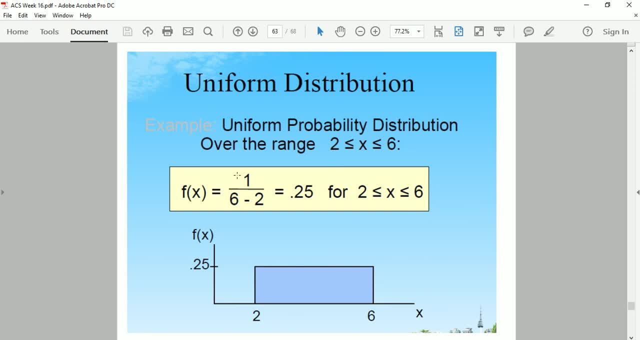 this is a function. a is 2 and b is 6, so f is 1 over 6 minus 2: 0.25. therefore x greater than equal to 2, less than equal to 6, so if you multiply them, 6 minus 2 is 4. 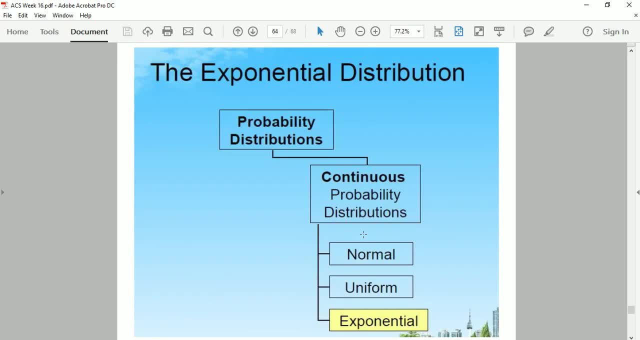 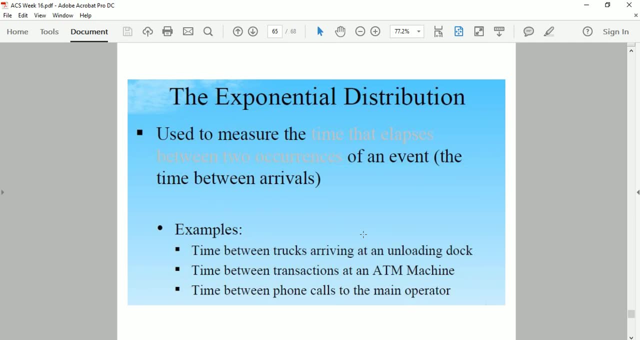 multiplied by 0.25, that will be 1. and finally, is your exponential distribution. exponential distribution it is used to measure the time that elapses between two outcomes of an event, like if it was a Poisson distribution. the time between the two events will be the exponential distribution. 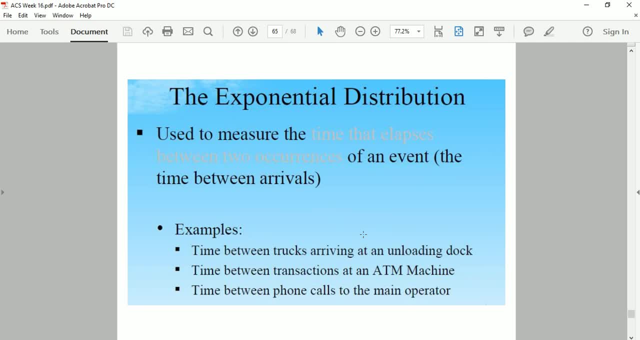 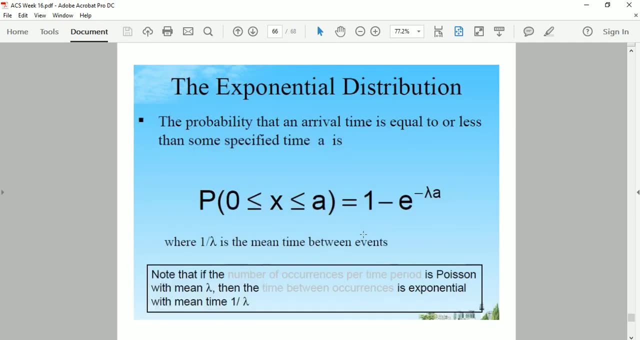 the time between the trucks arriving at an unloading dock. time between transactions and the ATM machine. time between phone calls to maintain the operator. now, how will we write this? the probability that an interval time is equal to or less than some specified time: a is p is x. less than equal to. 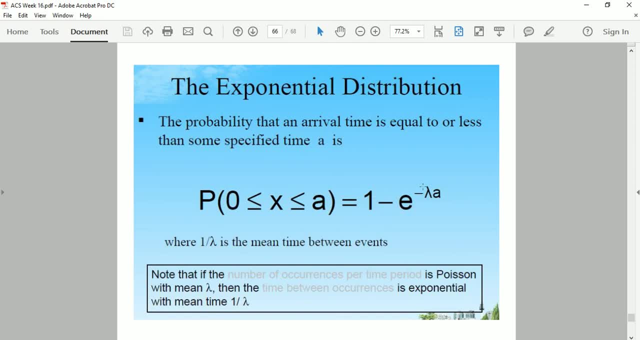 0 to a. so this is the formula 1 minus e raised to the power minus lambda a. now in this 1 over lambda is the mean time between the events: 1 over lambda. note that if the number of occurrence per time period is Poisson, 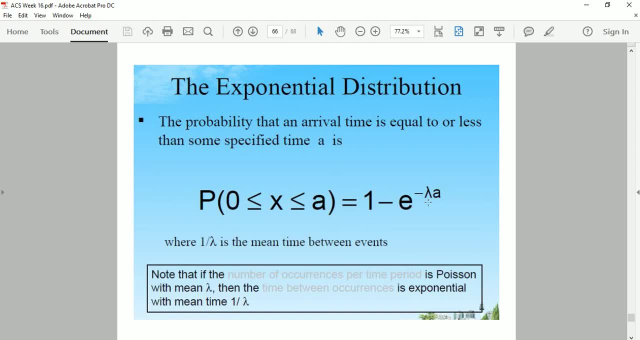 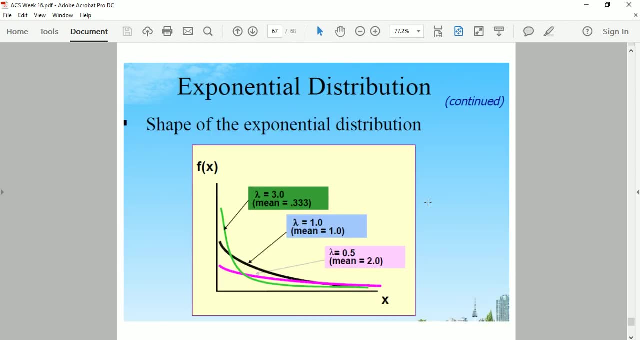 with the mean lambda, then the time between the occurrence is exponential, with the mean time 1 over lambda. this is a very important point. in the shape of the exponential distribution we are looking at what kind of shape it is. if lambda is 3, then its mean is 0.33. 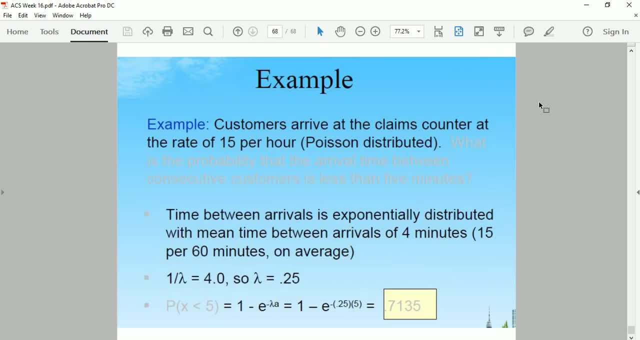 so this is the shape for 1 and 0.5. as you can see, and let's look at its example, customers arrive at the claims counter at the rate of 15 per hour, Poisson distribution and the customer- 15 customers are arriving in 1 hour. 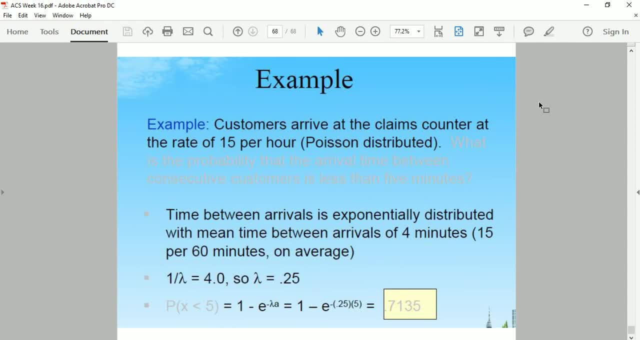 so what is the probability that the arrival time between the consecutive customers is less than 5 minutes? so we have calculated x less than 5. in this, the time between the arrivals is exponentially distributed with the mean value between the arrivals of 4 minutes. so 4 minutes will be the mean time. 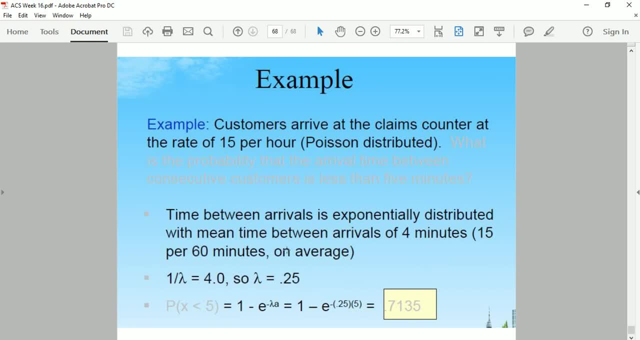 in the arrival 15 per 60 minutes, so on average it will be 4. 4 minutes will be the average, so 1 over lambda will be 4, because 15 is coming in 60 minutes. so the average value will be 1 over lambda is equal to 4. 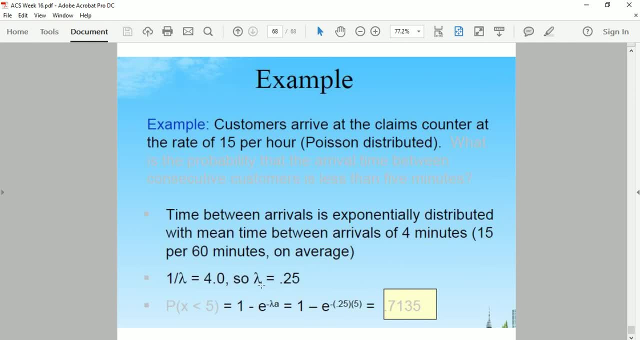 so every customer will arrive in 4 minutes. so 1 over lambda is equal to 4, so lambda is equal to 0.25. so the probability of px less than 5 is 1 minus e to the power minus lambda a. so in this, 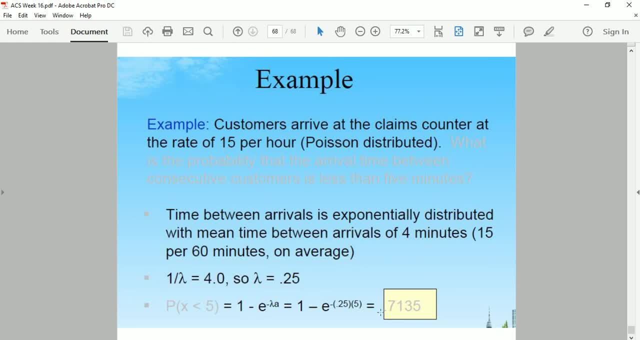 lambda is 0.25 and t is 5, so the probability is 0.7135. so 70% probability that in your 5 minutes what is the probability? that the arrival time between the consecutive customers is less than 5 minutes? so it is less than 5 minutes.